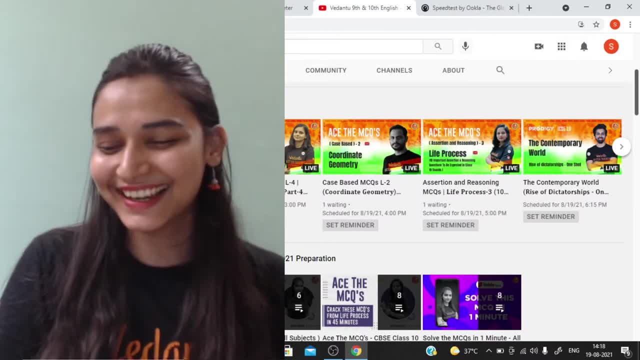 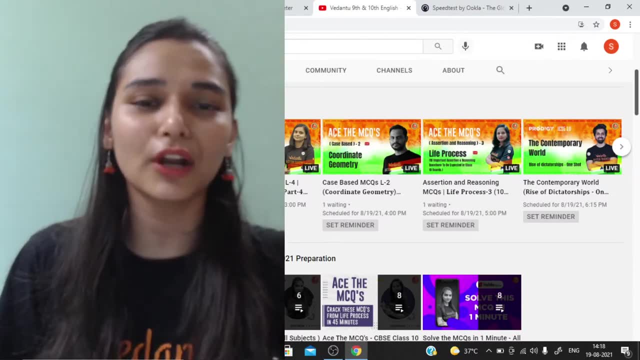 are you very smart and I see your profile picture. Okay, Hi, Surya, Welcome to Vedantu guys. So, beta, if this is your first session, then I would just say do not forget to subscribe To the channel. Vicky Shilpi ma'am always, you know, keeps on coming up with fantastic. 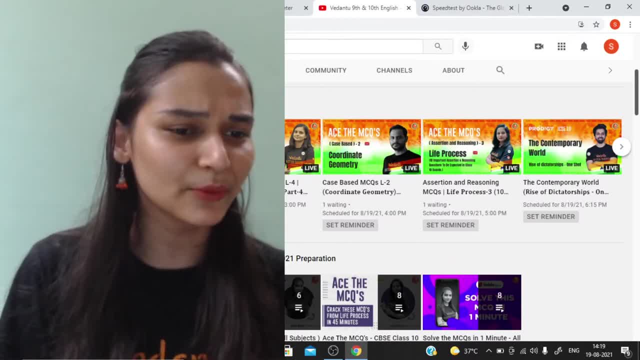 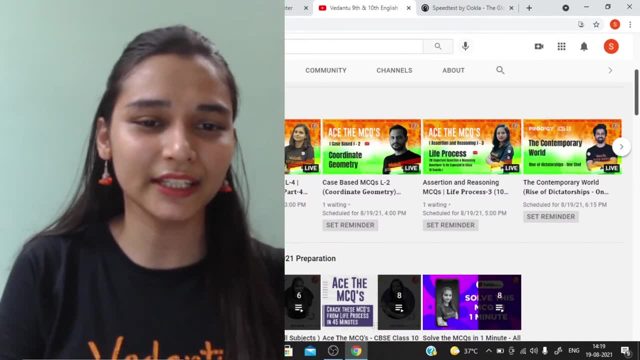 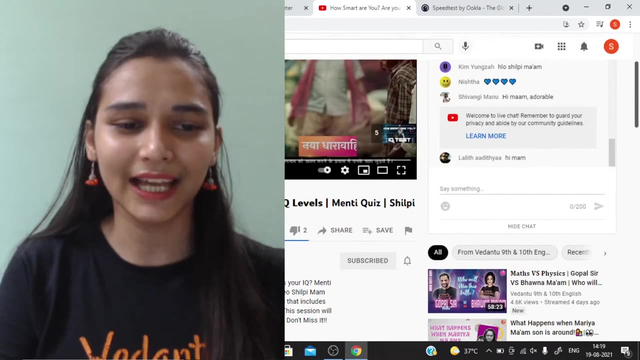 amazing ideas, So we have to do that. Yes, I can see some blue hearts. I need your support for that at the same time, and I can see so many blue hearts. Chalo Yaha par dekhte hai. Ma'am will mute herself and let me see how many likes we have achieved: 78 only Guys. 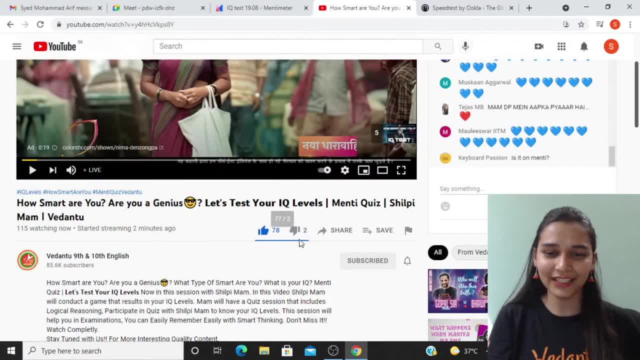 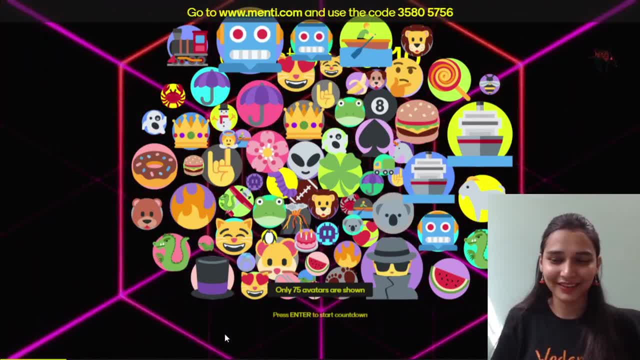 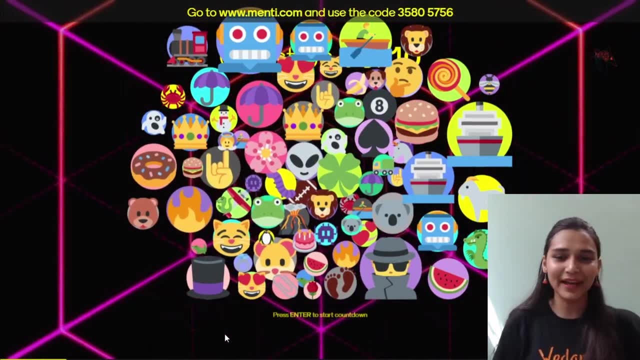 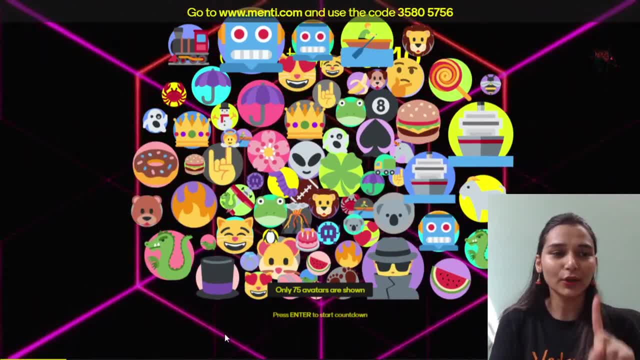 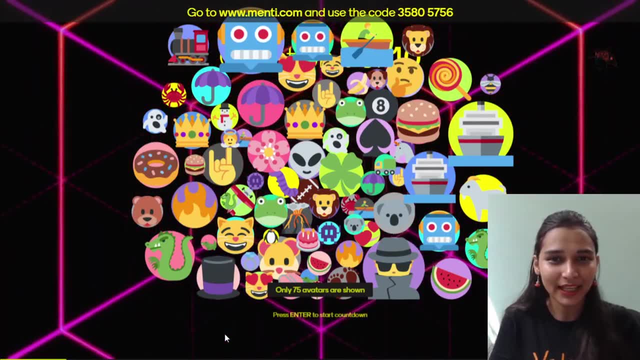 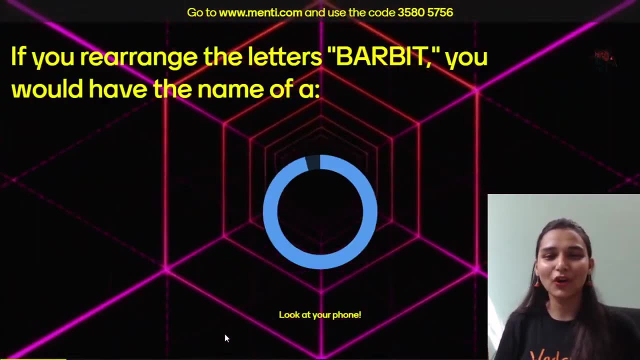 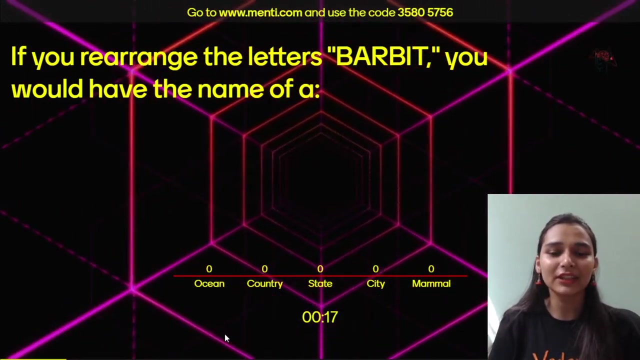 Okay, let's start. So first question is about to come on your screen. Get ready all the very best and remember time and accuracy. They both are going to decide that. Okay, precise, You have to be precise. First question on our screens. Very easy: If you arrange the letters B-A-R-B-I-T, you would have the name of an ocean, a country, a state, a city or a mammal. 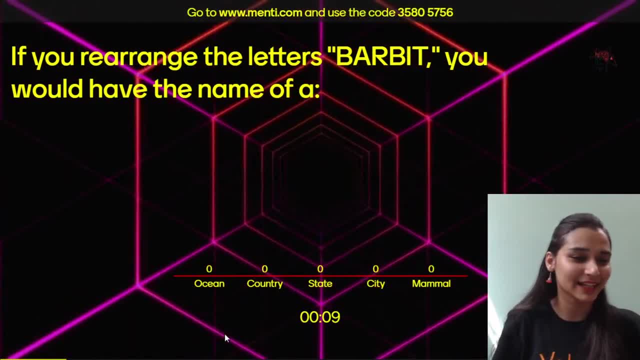 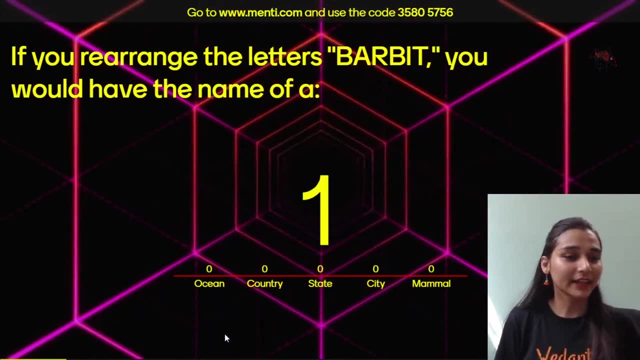 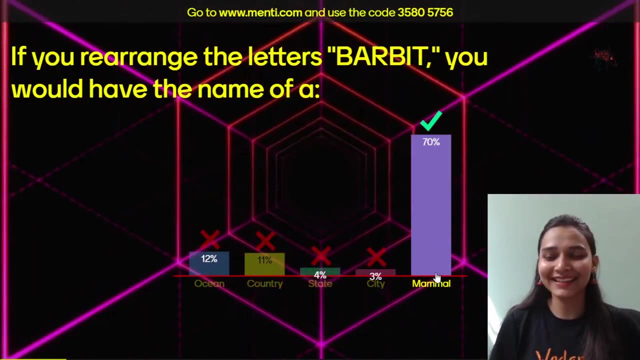 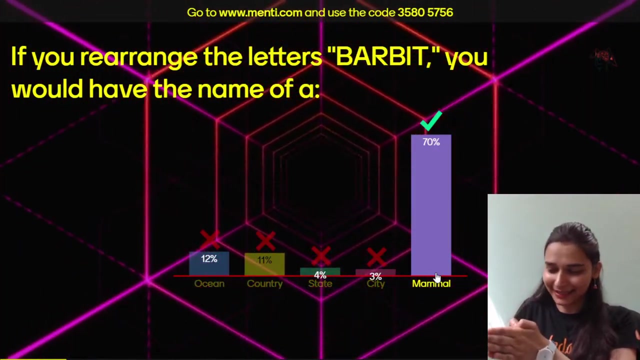 You get only 20 seconds Now. you have to be fast, as fast as anything. Anitha beta, the code is 35805756.. Angel, try it again. I have misclicked. Oh my God, That is so amazing. Standing ovation- This is a normal clap. I will give you a loaded gun clap at the end of the session. Let's see what so special is coming in that, Okay, Yes. 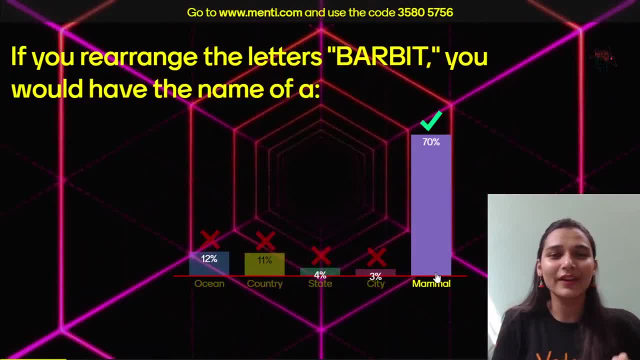 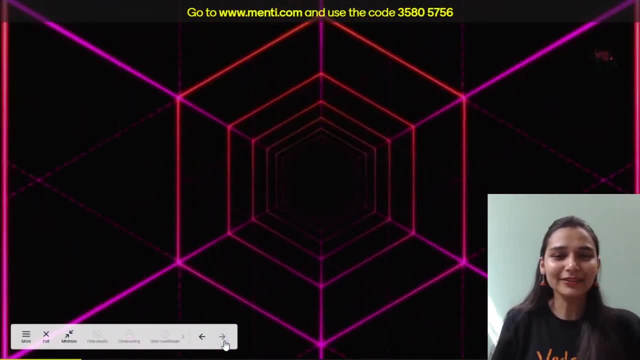 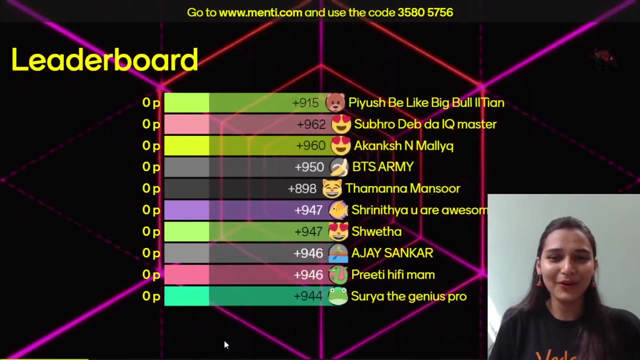 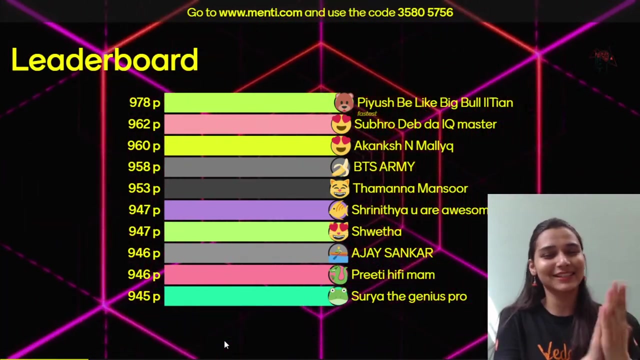 Okay, so that's amazing. If you are a mammal, you know that you will get a word: rabbit. Rabbit is not an ocean, not a country, It's a mammal. So that was a correct answer. Let's go and see our first leaderboard and what my students have done in their IQ. Oh, oh, oh, oh, I can see like: okay, Piyush is fastest Piyush. well, I must say that beta, Amazing, Big bull, IIT and wow, All the very best Piyush. 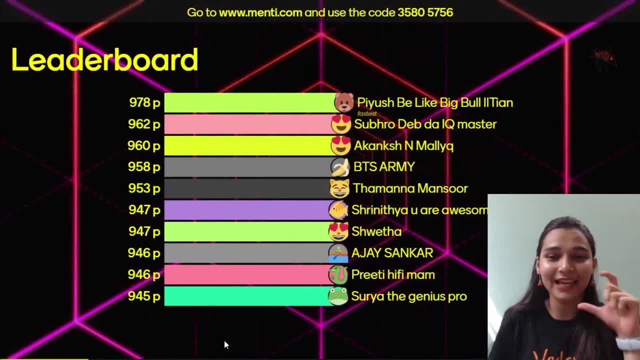 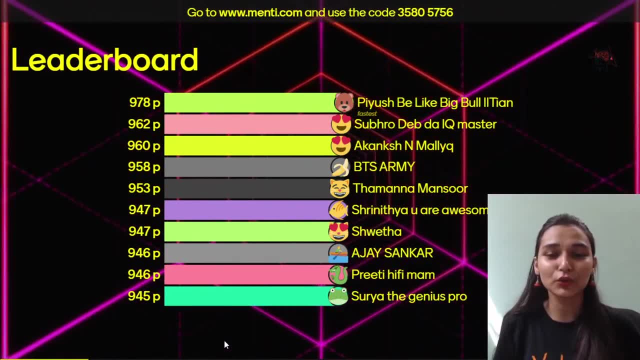 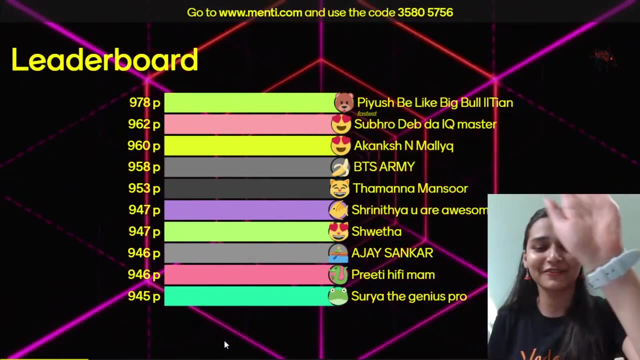 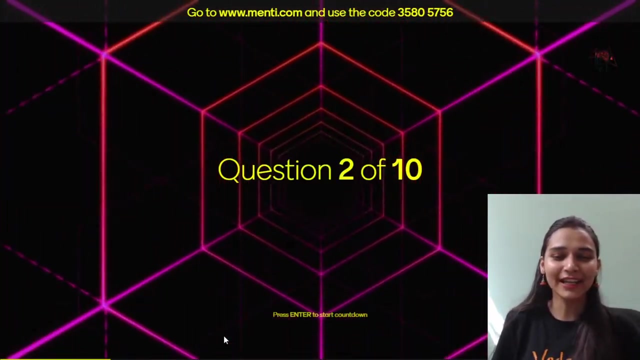 Second. That's also amazing, And the point difference is very less Akanksha. only two points difference in the second and third. That's amazing. BTS Army. then we have Mansoor there, Then we have Srinithya. Thank you so much. Piyush Shweta is there, Ajay Preeti- high five And Surya the genius pro, Just like Vedantu pro subscription. Okay, let's go to the second question. Join in again. I see 165 students in the mentee. 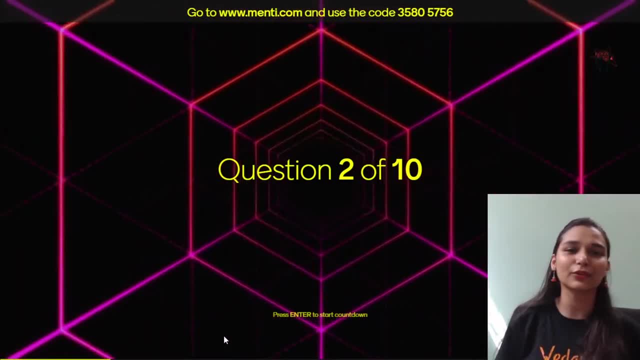 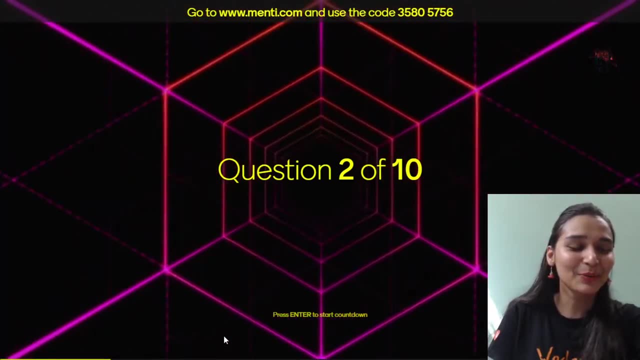 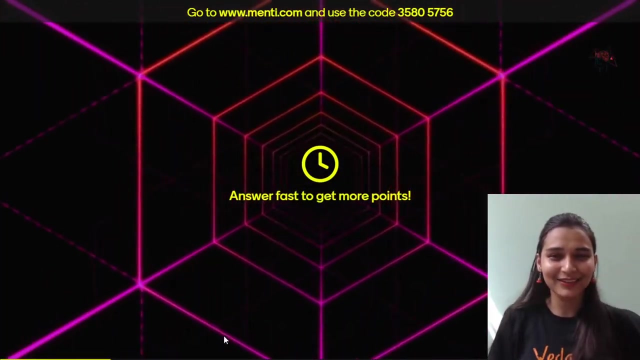 Yes, and in the live chat as well. So have we achieved 200 likes? No, ma'am, you are getting too greedy. I will dislike the video. if you do it this way, 126 likes are done. I have trust on you. Second question: all the very best And remember IQ test. 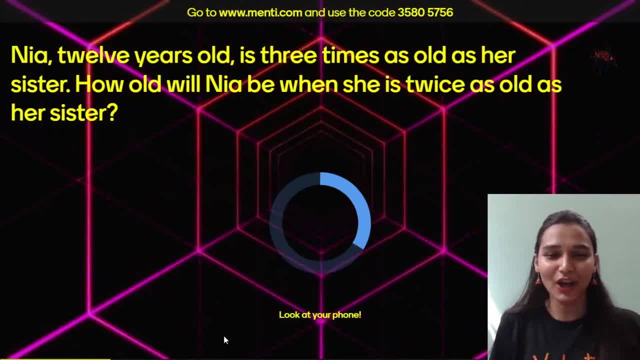 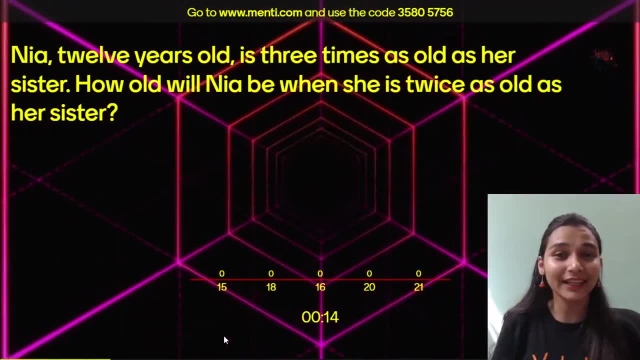 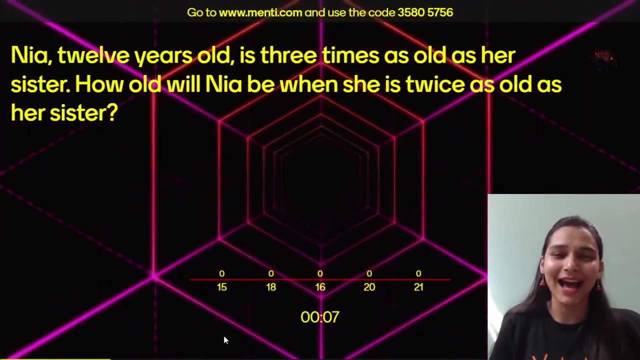 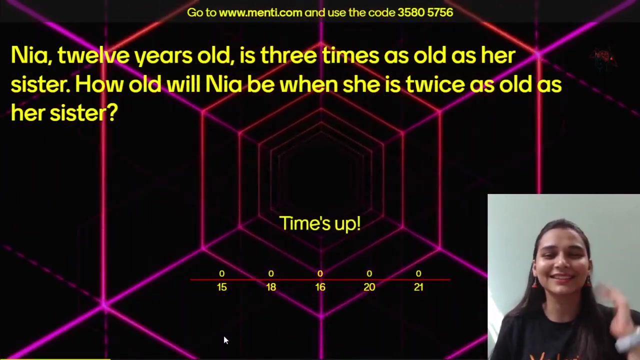 Shilpi ma'am is not just here for chemistry. Come on, I can teach you other subjects as well. Not really. Shilpi ma'am is as old as her sister. How old will Mia be when she is twice as old as her sister? Well, I am going to call your maths teacher right now. I guess I should call Harsh Priyam sir and ask this question from him, Isn't it, And give him a time frame of only 20 seconds. 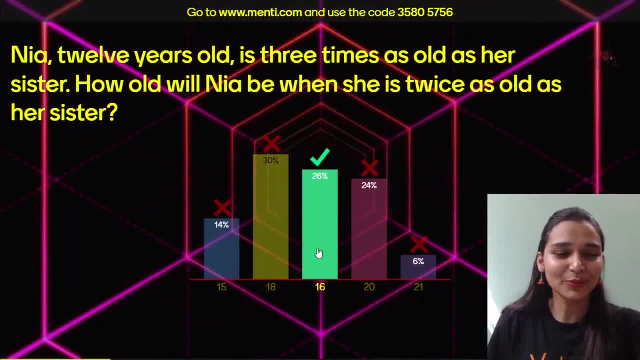 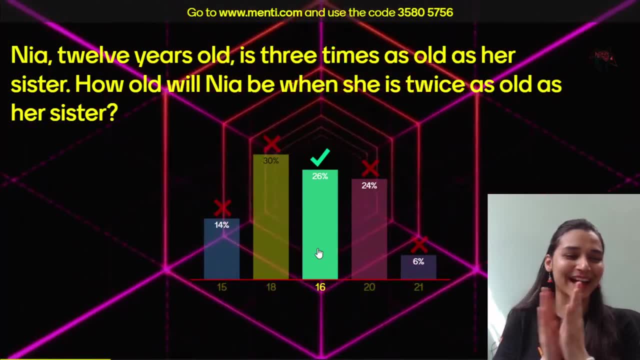 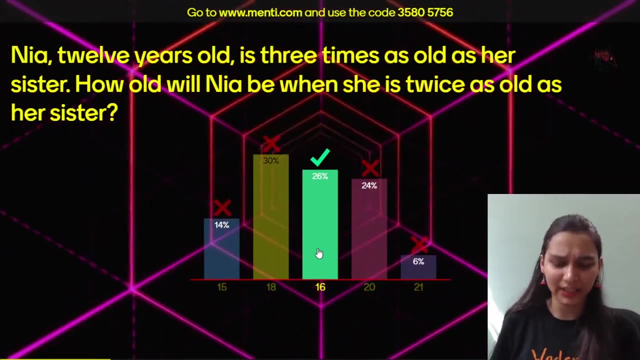 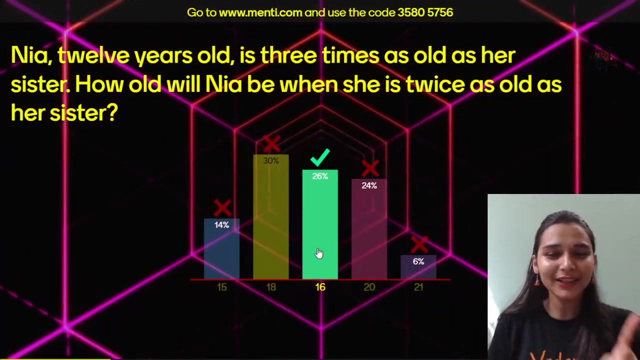 Hmm, 26% students. The odd went out, and that's awesome. Shashi Raj is saying: ma'am, teach maths. I cannot teach social studies Maths, toh. still, I can think of teaching you. Yeah, I should call Gopal sir and ask this from him, Isn't it? Well, the answer was 16.. Now you have to solve this in the comment section, All those who have done it right. Okay, That's awesome. 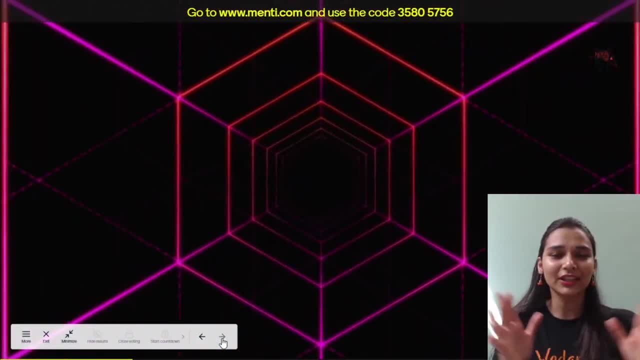 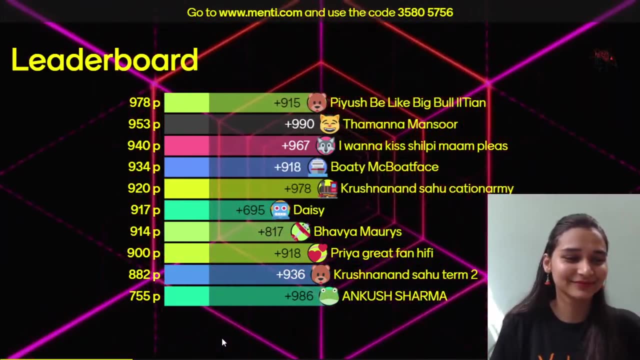 Chalo. let's go to the third question on our screen. You still have a lot of chances. Now take a screenshot of the question and think: yeh kese galat hua. Okay, Yes, Tejas, I know right. 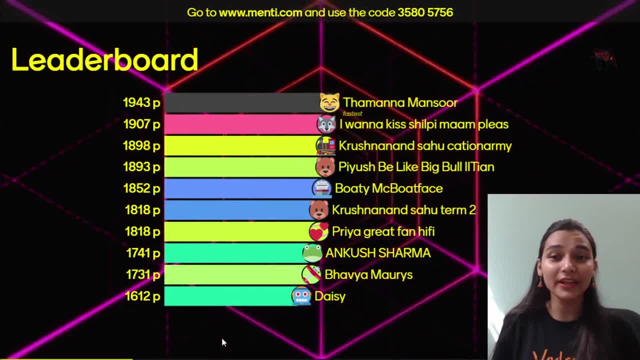 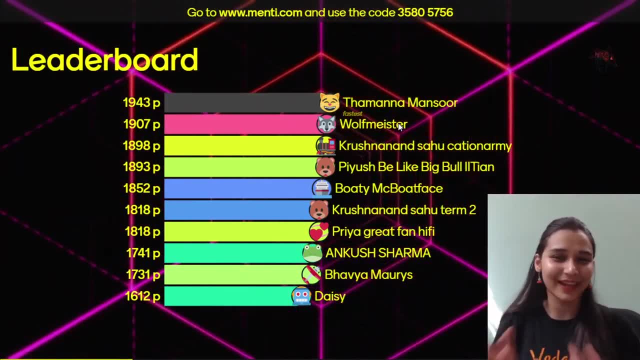 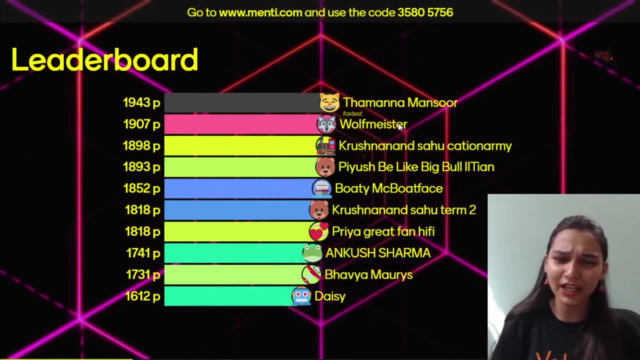 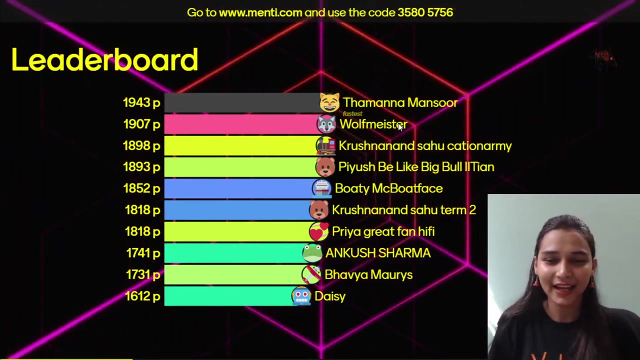 Janki joined in the session again and Thamanna Mansoor has changed the. oh my god. The first position is taken by Thamanna. now, That's amazing. And Wolf is there with us. Krishanand, Piyush Boti, then again Krishanand Sahu, term 2.. Okay, the first one, Krishanand, is from Kitain Army. Okay, I see that. Then Priya, Ankush, Bhavya and Daisy. I see some new names. Guys like you have really got the hang of it. 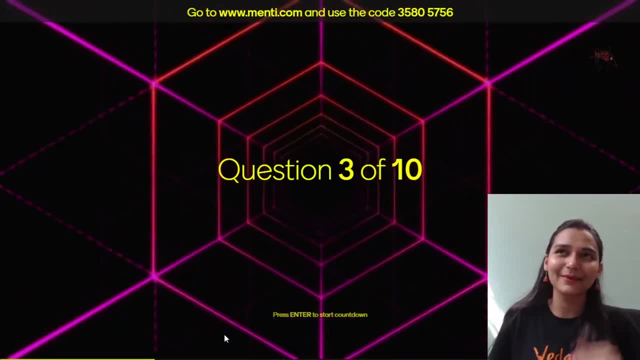 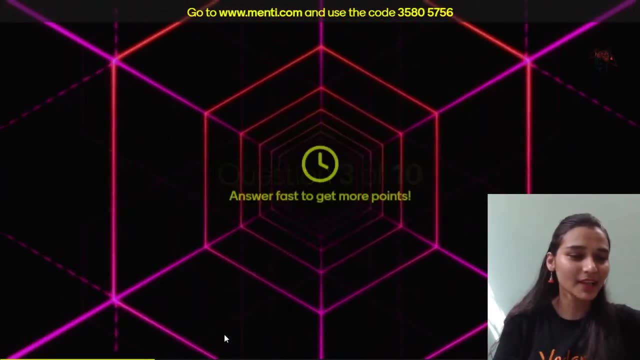 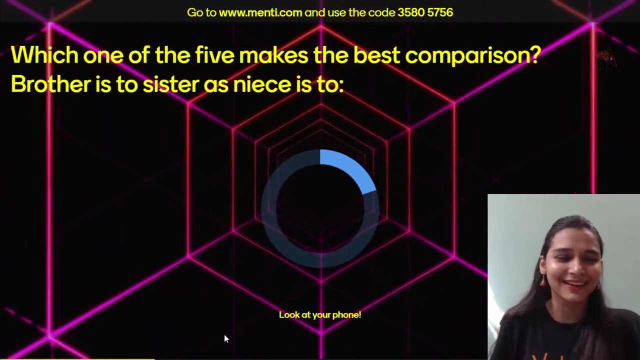 Some amazing IQ level. Muchhe bhi dedo, yaar thoda. At times I act so dumb. I really need that, Yes. Third question: Sneha, happy birthday to your friend Akshay bida. Akshay, God bless you. I guess Akshay ka rose birthday nahi hota. Okay, Which one of the five makes the best comparison? 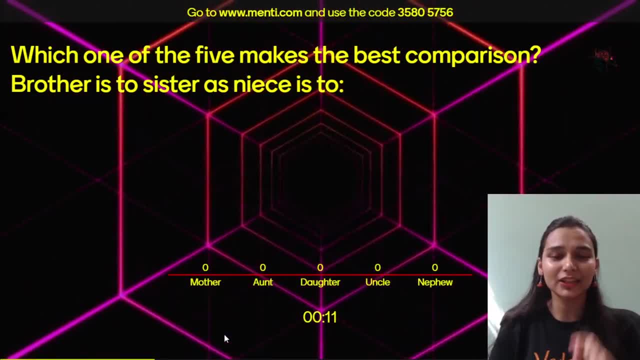 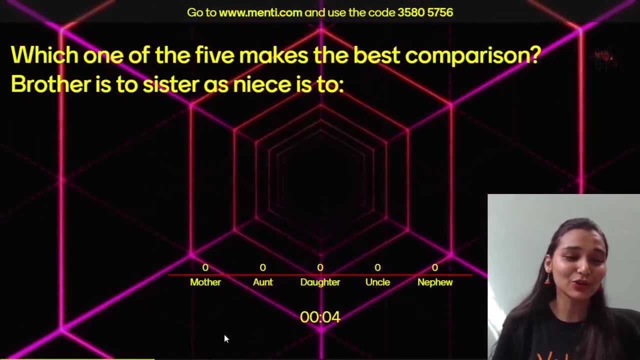 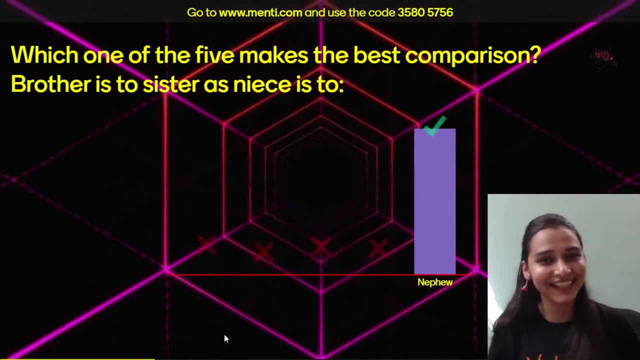 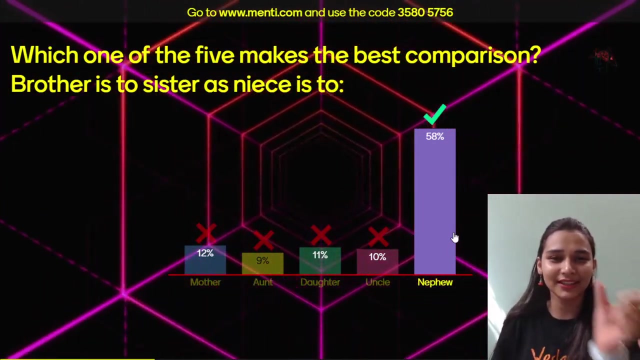 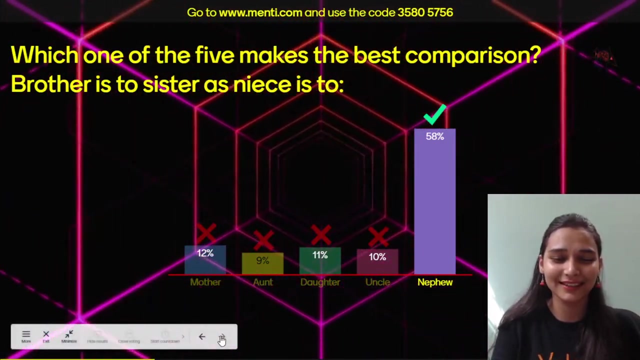 Brother is to sister as niece is to mother, Daughter, uncle and nephew. Yes, Shashi bida, how to join my batch, You have to apply my coupon code SKA PRO in the Vpro subscription. Thik hai, You can apply that. Shilpi Kaushik Army Pro- SKA. Okay, amazing, That's nephew. Brother is to sister as niece is to nephew. Like lot of you have got it right within Mother, kaise hua beta Exams is like. Yes, ma'am, That was a misclick. 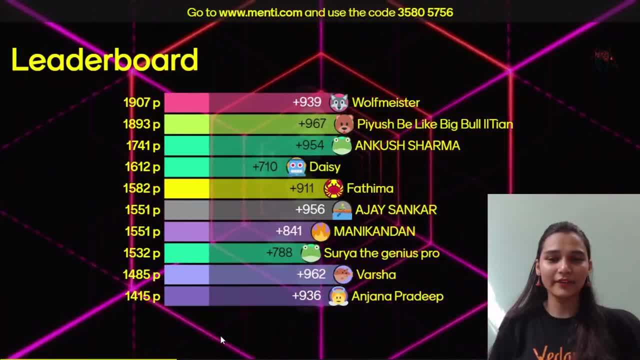 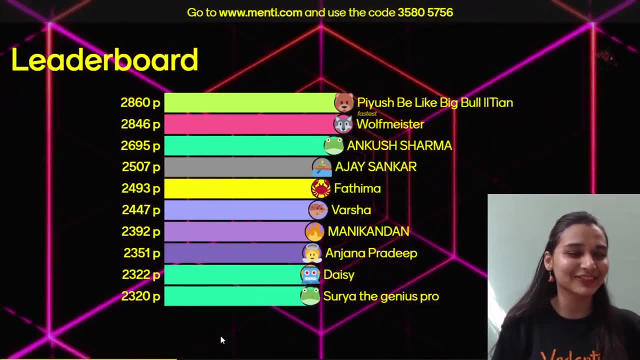 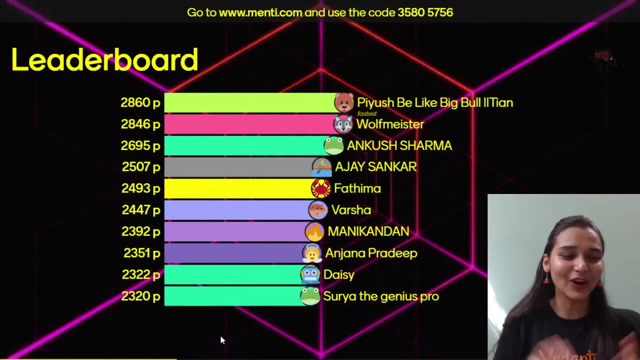 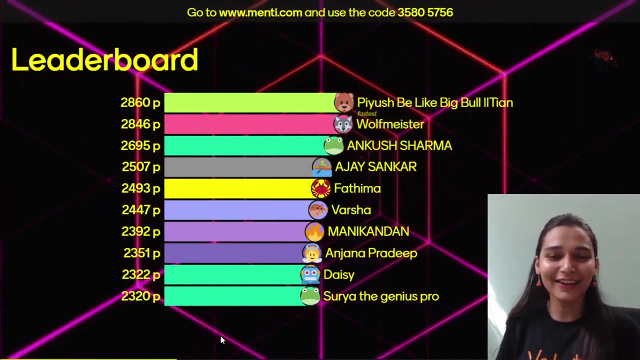 Okay, let's go and see On the top we are having, Piyush again has grabbed the first position. I can see there's actually there's a huge competition going on. Yes, Janki, it's a combination of all the questions. Yes, Yes, they just right. Piyush again was Mr. Very close competition you people are having. 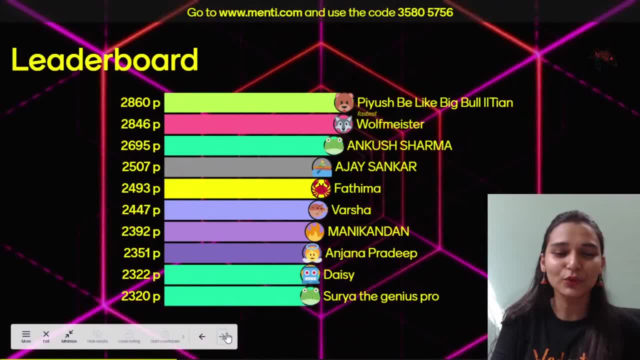 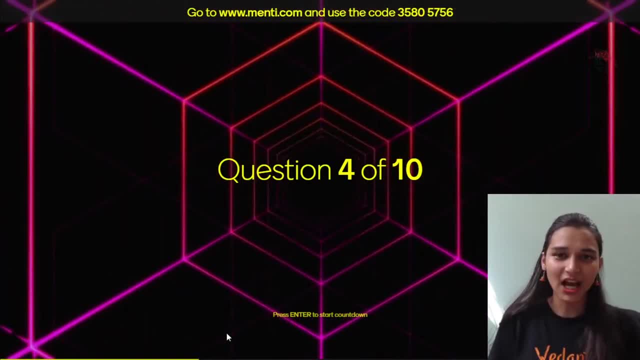 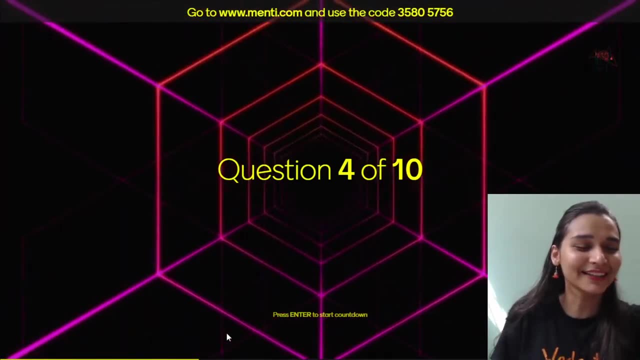 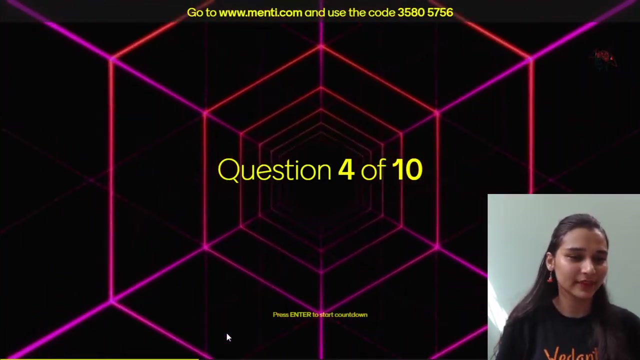 Have gotYou can have I the person Alisha, Manikandan, Anjana, daisy and Surya again making a position on the leader board. that to not in a normal session, guys. That's IEQ level Check. 4th question: You all are ready? Yes, Okay, so I want to know the energy in the chat box. Come on. 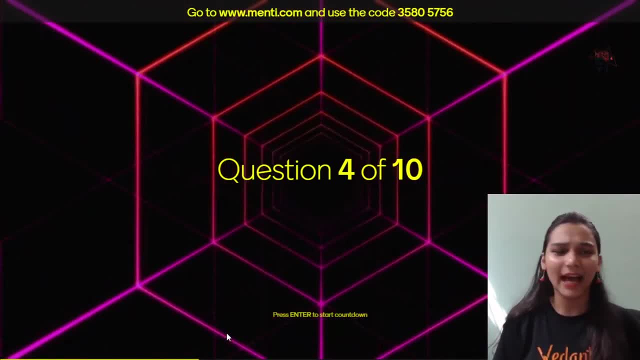 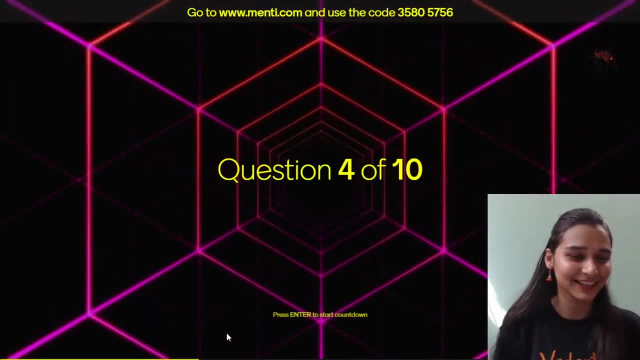 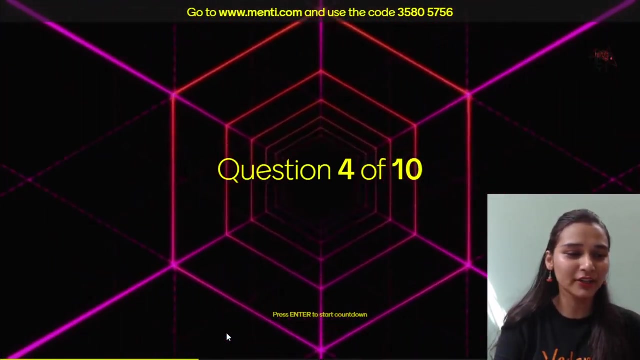 How you express it, box, how you express it, I don't know. yes, you know, ma'am is an emoji kind of person, so I always like to see lots of emojis. yes, thank you, Shashank beta. thank you so much, okay. fourth question on your screen and there we go. 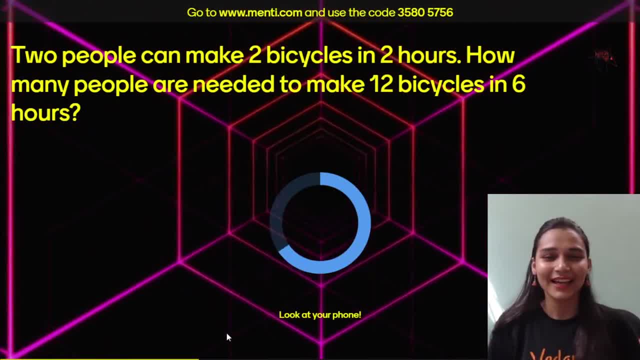 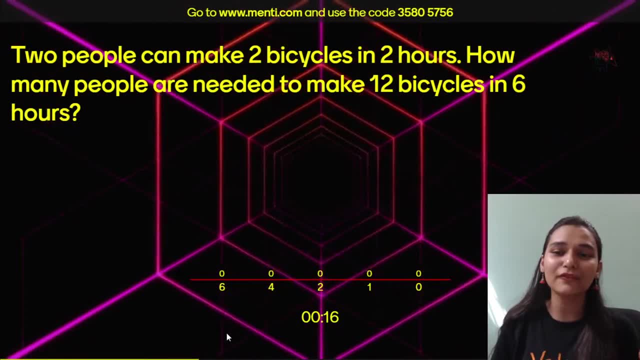 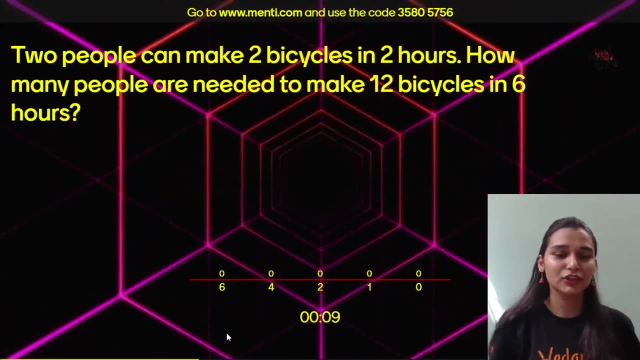 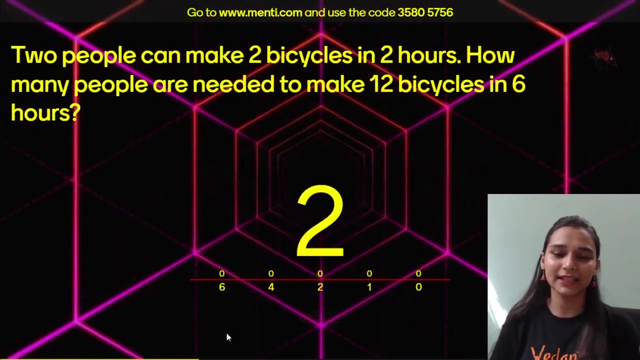 okay, Priyal, it's okay, so attend this. two people can make two bicycles in two hours. how many people are needed to make 12 bicycles in six hours? yes, come on. two people can make two bicycles in two hours. how many people are needed to make 12 bicycles in six? 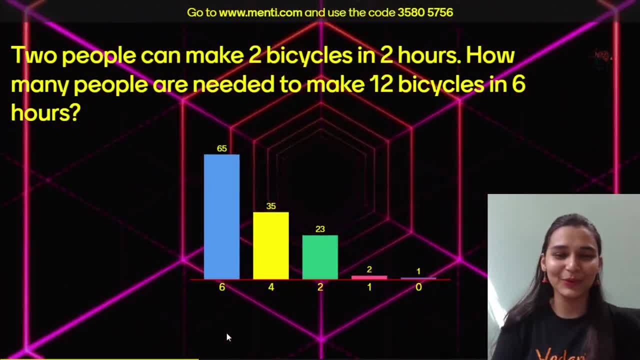 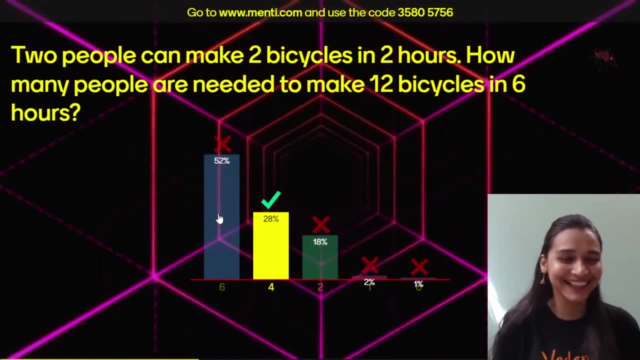 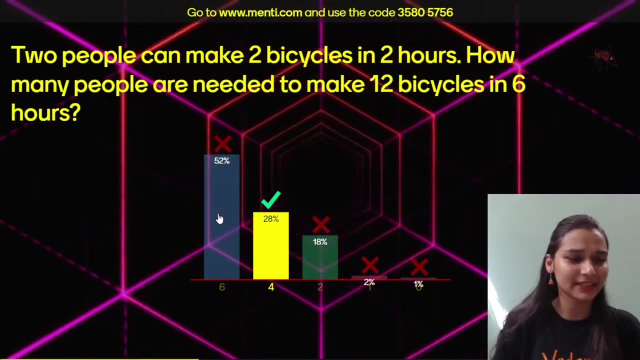 hours, I don't know like how. oh oh, oh, oh, not bad, that's amazing. 52 percent have marked it wrong. I thought that's right, beta, beta. correct answer is four people are needed to make 12. that would be six. na ha, A is the correct answer. A is the correct answer. like that is marked wrong. 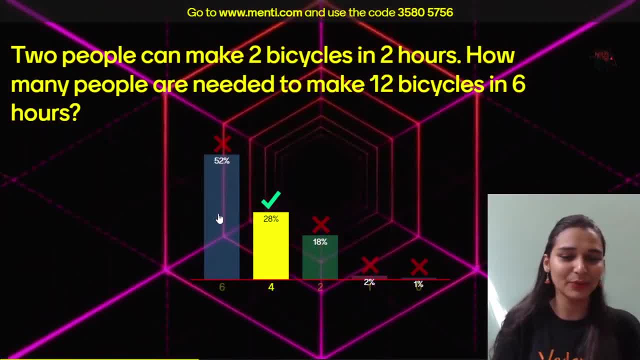 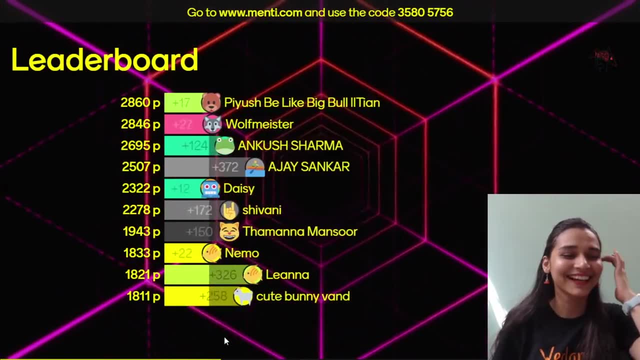 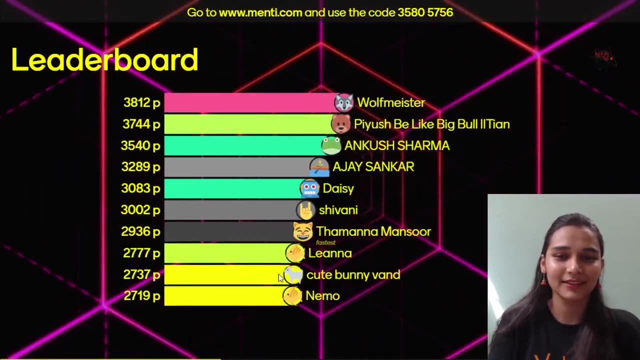 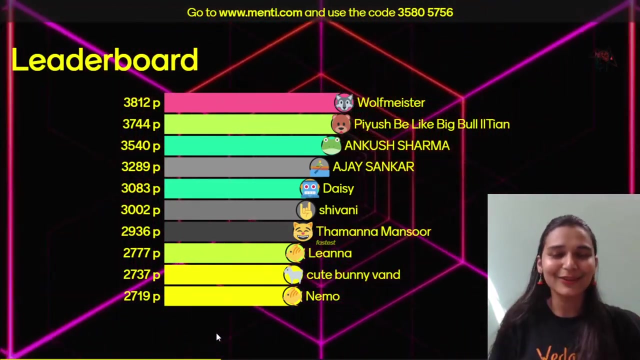 still amazing. we will check it. okay, we will make it clear, don't worry, let's go and directly jump to the next one. yes, okay, so wolf. again Ma'am has maintained the position. It means even ma'am cried out in math question. I didn't saw that question. how many people can solve it in? 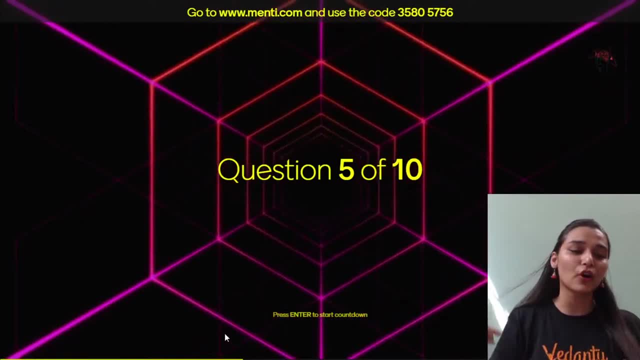 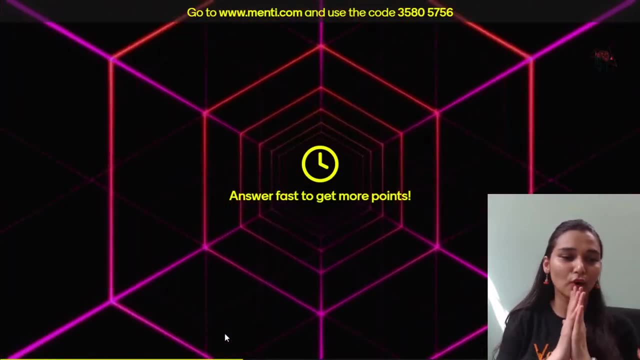 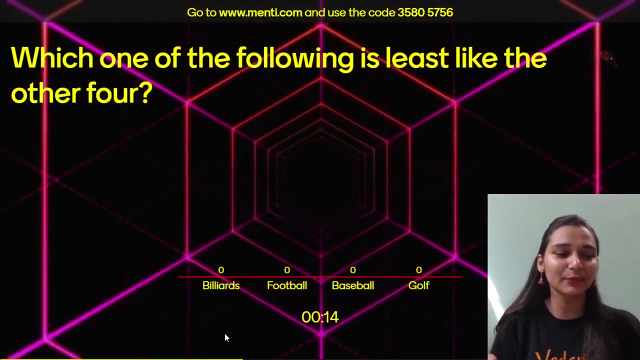 how many days and hours? lets go to the next one. Sadeen beta, join in the mentee again. yes, okay, let's complete the fifth question on the screen. just go and see it. which one of the following is least like the other 4? other three? uhh, basically this will happen. 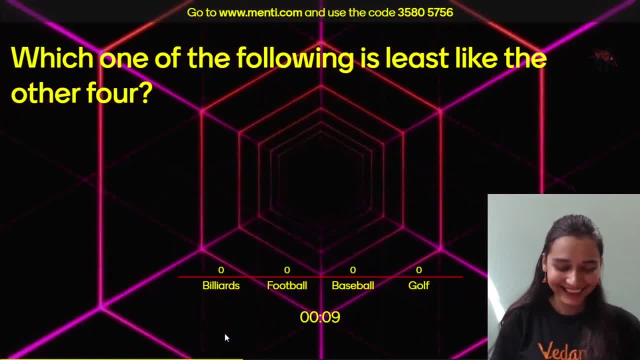 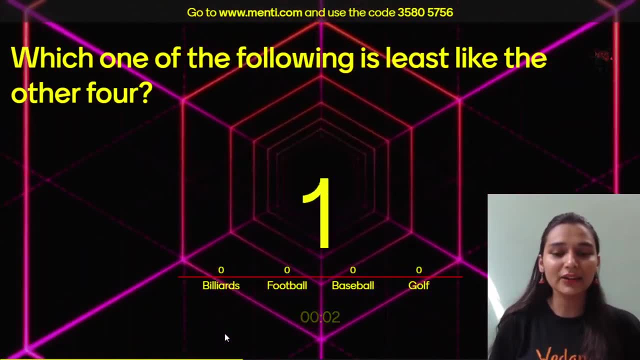 no, harsad had not come beta, then only he will be sorted out. Wahi toh baat hui na. we will call Harsh sir, for that, isn't it? Isko karo, you have billiards, football, baseball or golf. 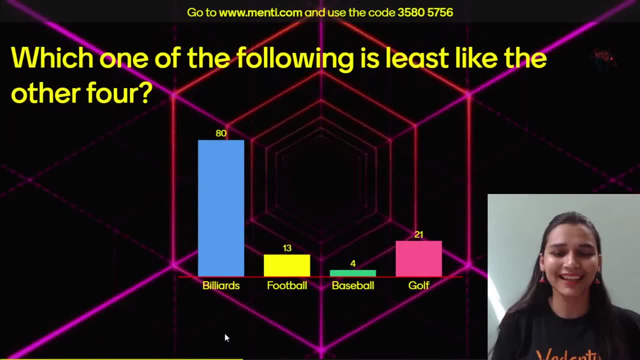 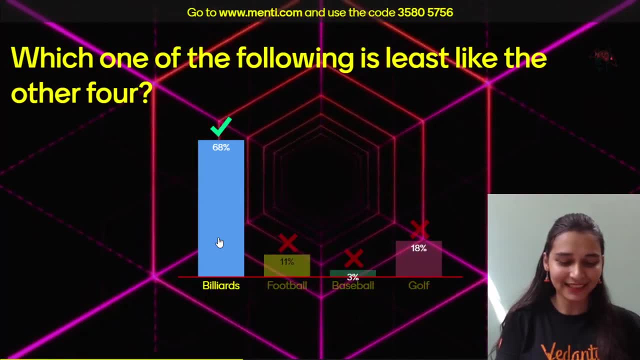 Which one of the following is least like the other three? You have done cheating. Come on, I showed you the answer, isn't it? Kitne logon ne cheating kiya iske liye, Haan ma'am, I don't even know what is this game- billiards. 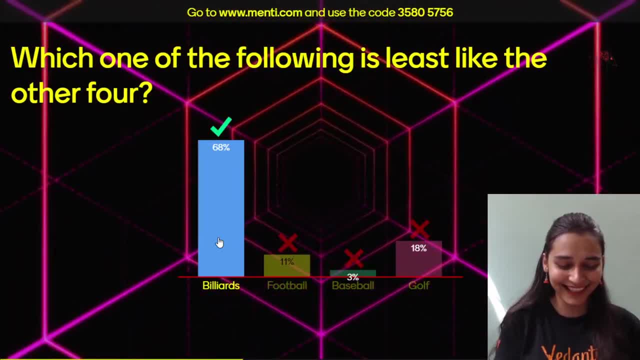 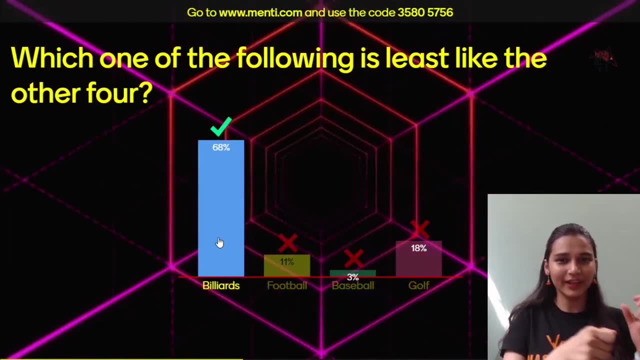 Haan, I know I know right Koi baati. so billiards is like wala game. hoda hai Jisme. you have a ball and a stick. Stick ke saath balls ko hit karna hoda hai. Okay, and that is an indoor game. 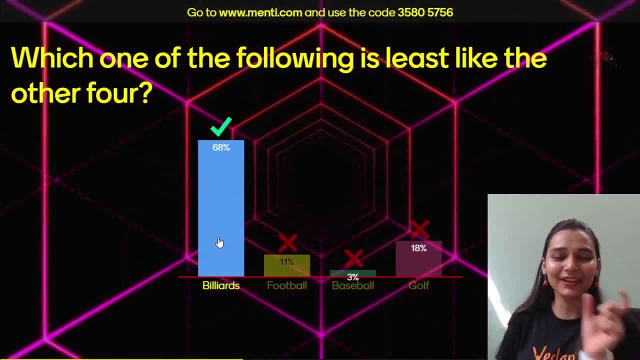 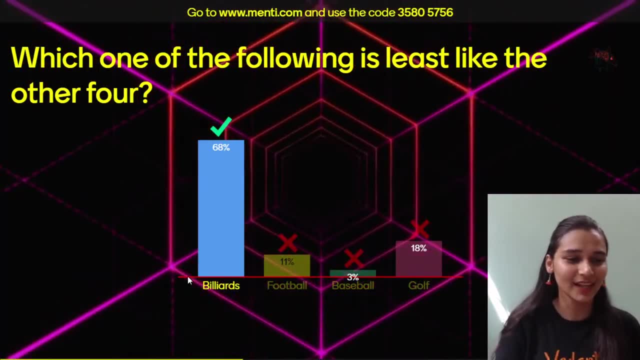 I know that that's an indoor game: Football, baseball and golf. they are the outdoor games. Yes, haan, pool, you can say Shashi, that's right, Arjun, same hair, beta, mutual feels, don't worry, Don't worry, let's go and see the leaderboards. 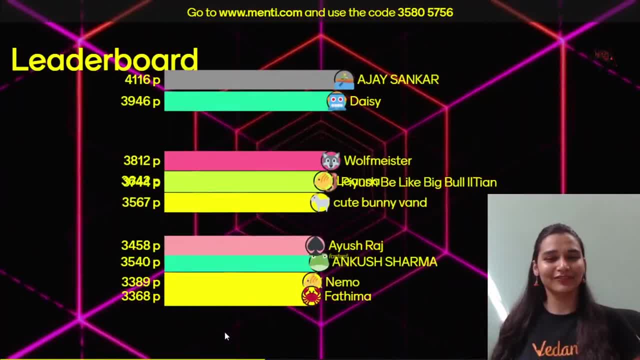 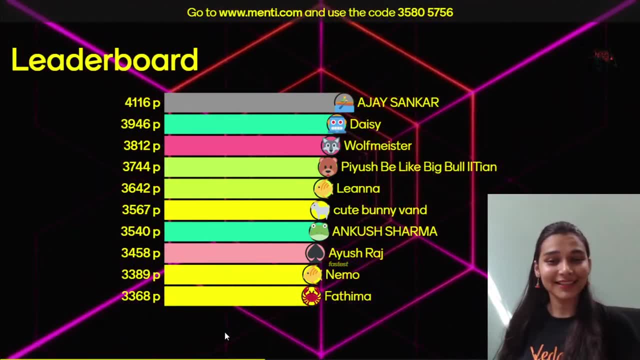 Piyush, Ankush and boss be like arey, yeh kya ho gaya. Ekdum se saari duniya palat gai. Ajay on the top now and Daisy second- Daisy has actually climbed up. Wolf and Piyush on the fourth now. 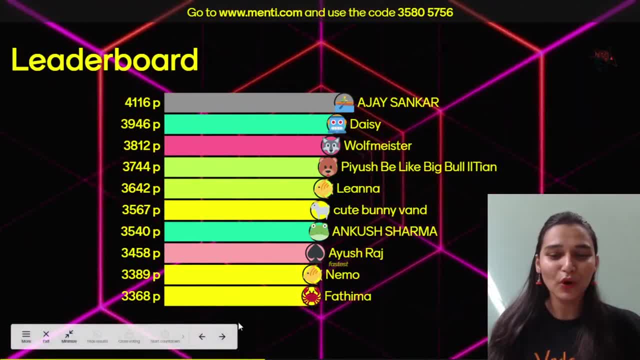 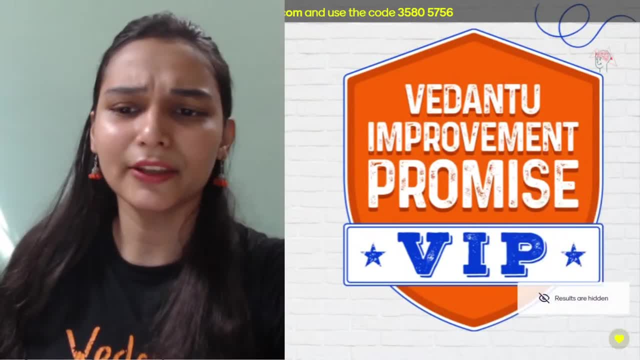 Then Leda Cute Bunny Ankush, Ayush Nemo and Fatima. Ayush was fastest this time, That's awesome. Okay, so this point, ma'am is just telling you one thing, That if you want to be a part of Vedantu's regular sessions, 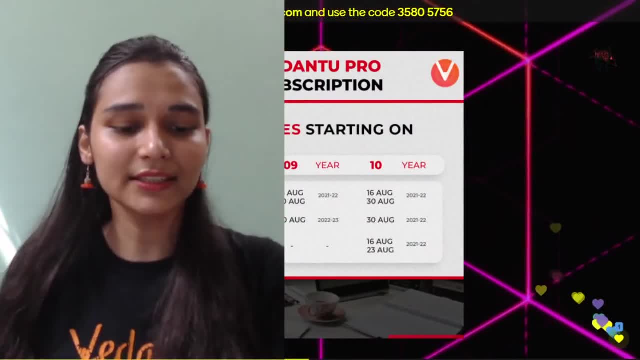 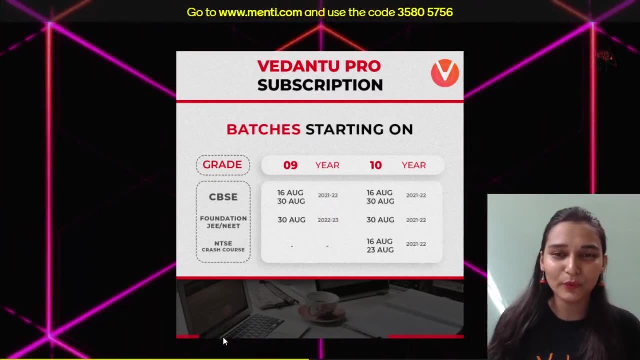 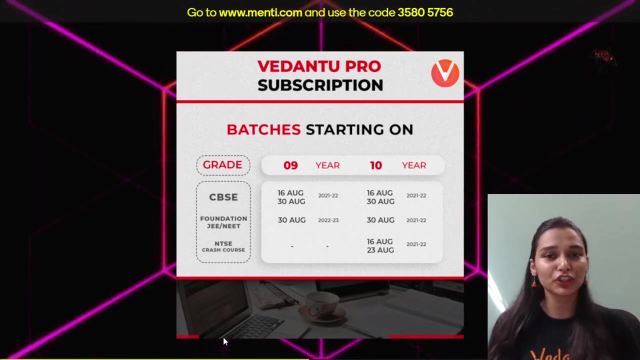 Then you can apply now, Because the new batch is starting from 30th of August, right? So if you wanna complete entire term 1 and term 2 syllabus in just one month, Then you can take the enrollment for this upcoming batch, Which is scheduled for 30th August. okay. 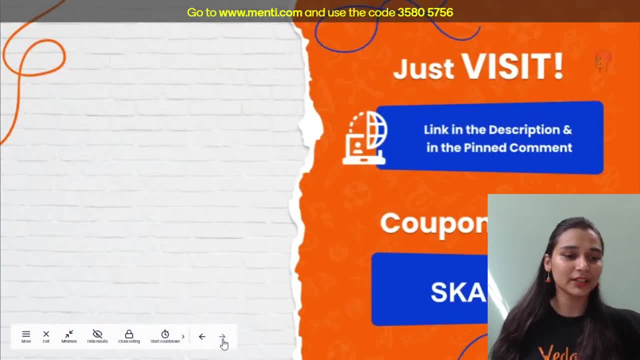 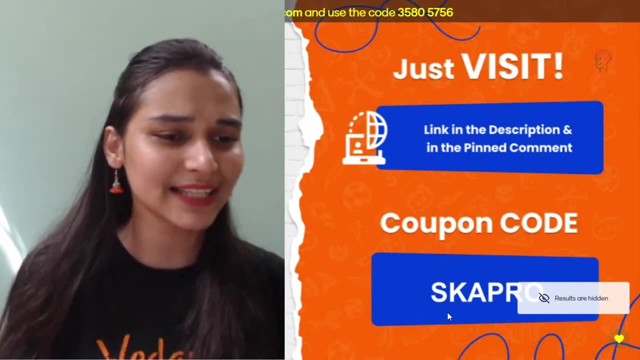 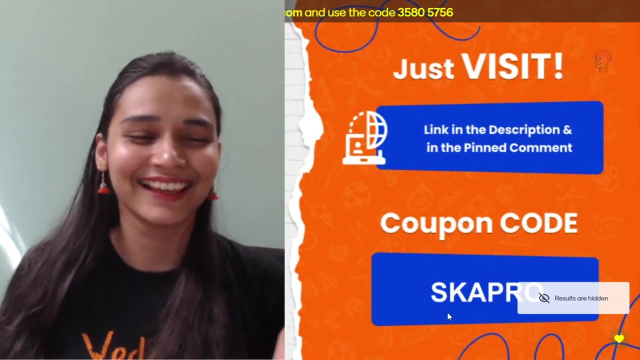 So all you have to do is go in the description box of this video. You will get a link, And then you have to apply a coupon code That is SKAproof. I guess that is it. It is clear to you, isn't it? Yes, Nikhil, that is not SD, that is SKA. 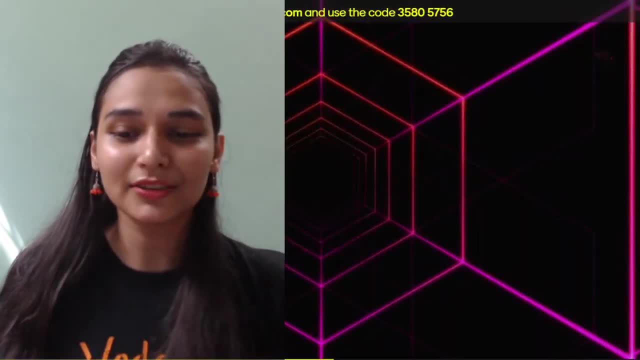 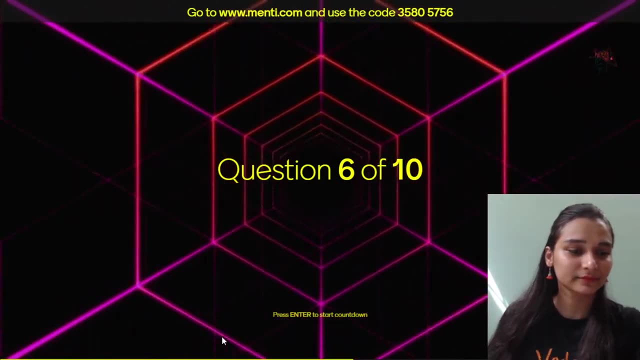 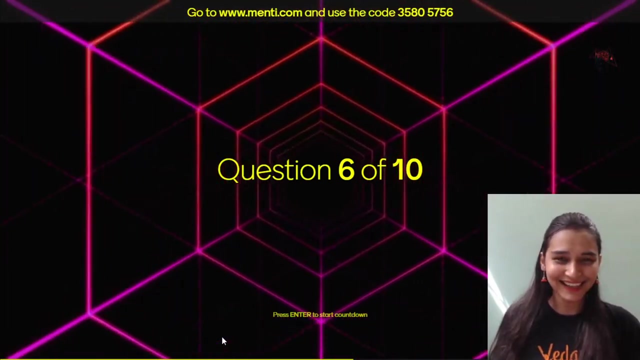 Yes, Okay, let's go to the next question on your screen, And there we go. Sixth question: everybody is ready? Yes, Yes, Janki, you said it right, Janki, you applied it. Okay, let's go. Sixth question on your screen, and there we go. 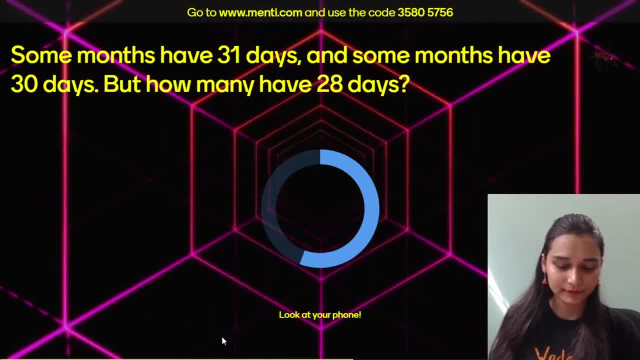 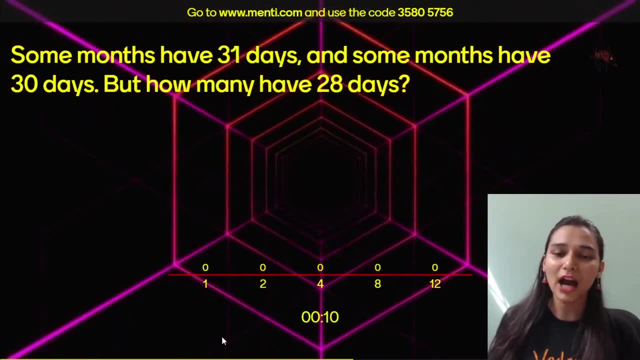 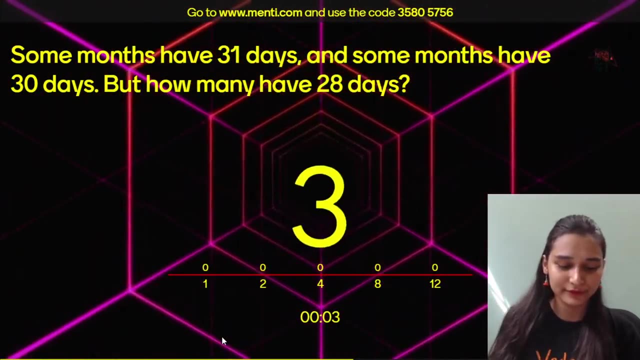 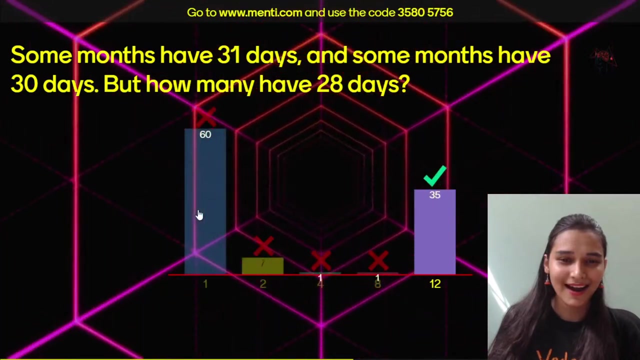 Some months have 31 days and some months have 30 days. But how many days? how many months have 28 days? 1,, 2,, 4, 8 or 12? Yes, Now this one who has done A. So you guys tell me. 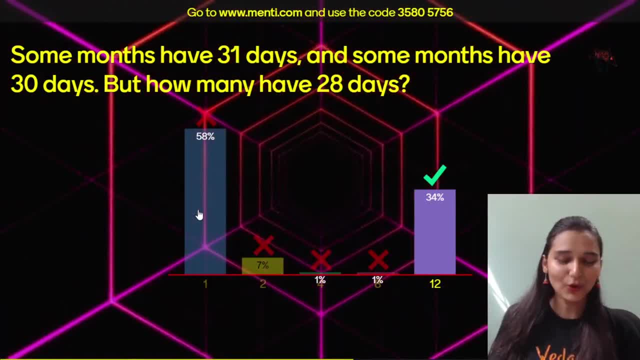 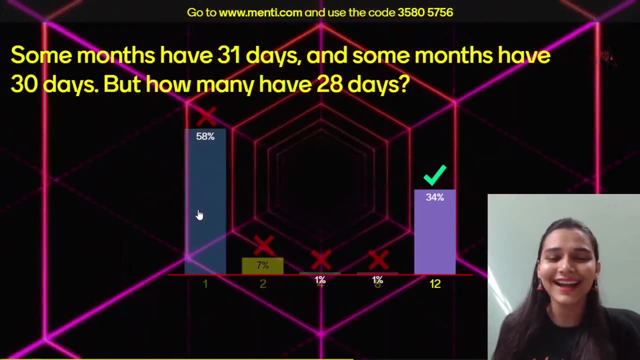 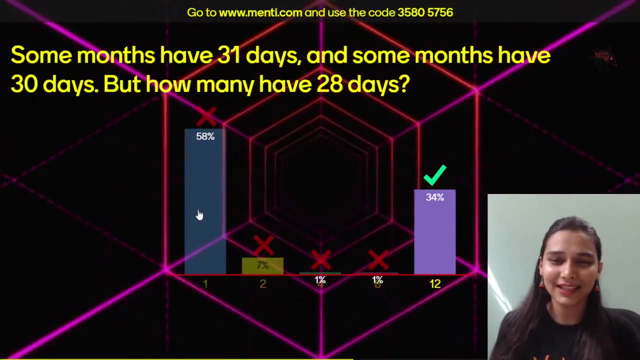 So you guys tell me one thing You have thought of February, isn't it? You thought that in February only there are 28 days, But all the months are having 28 days, guys, Come on, Not in August 28 days, January has 28 days. 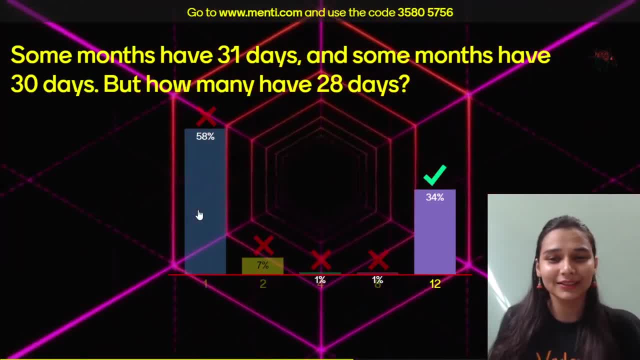 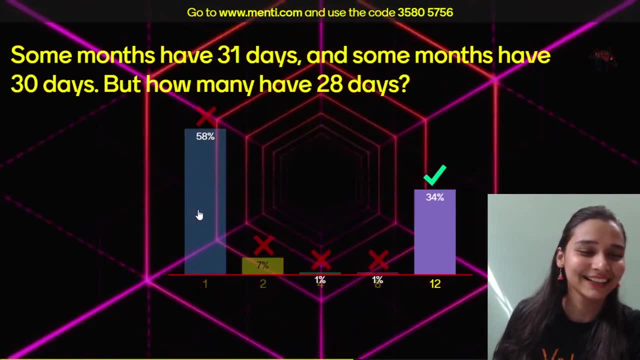 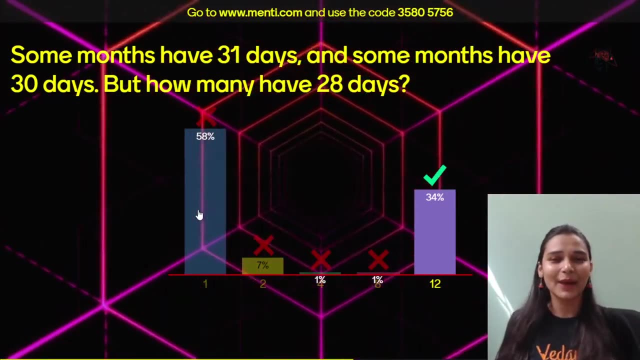 February, then March 28. Every month is having 28 days. That is what we call as IQ. now, Okay, so you have to think that way. Yes, Warriors, you are having a bad network in Kashmir. That's okay. Sometimes bad network happens everywhere, Even in Haryana as well. 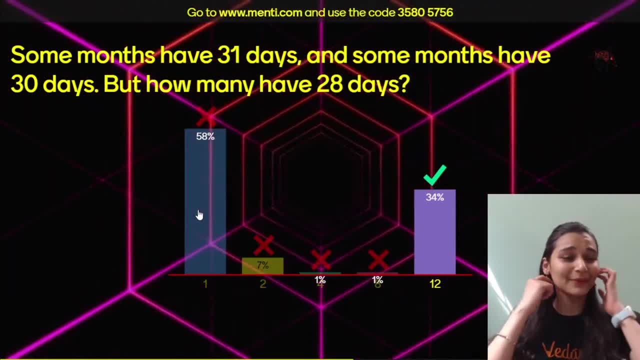 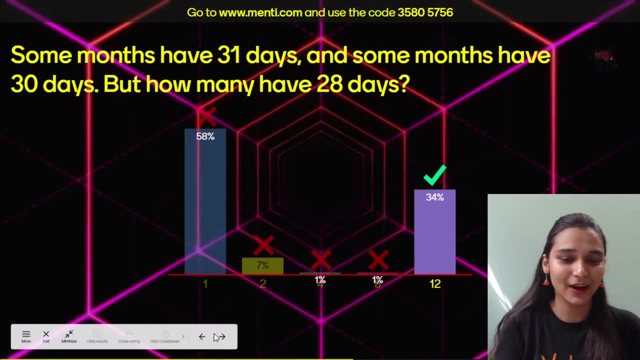 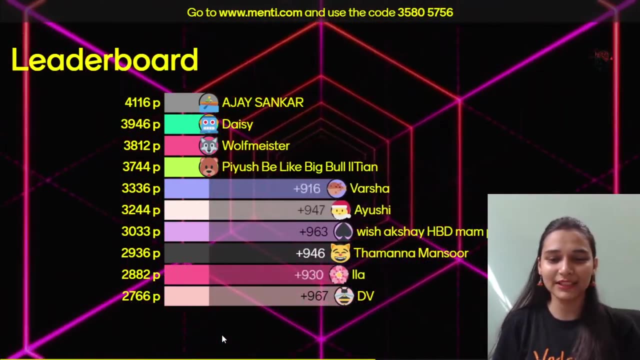 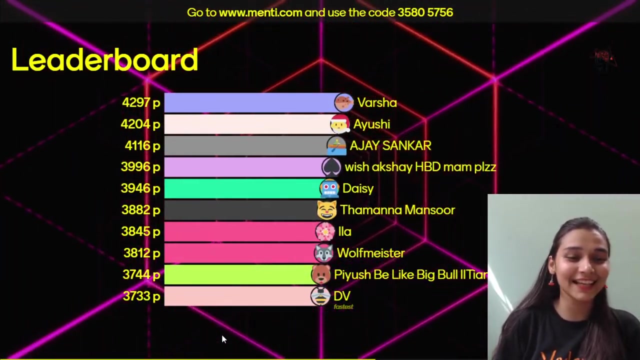 Just take a chill pill, Shashi. my micro course is also starting this month, only Next week. Yes, Okay, So 12,. all the months are having 28 days On the fastest fingers list. I wanna see how much the positions have changed. Hmm, Yes, Yes, Nikhil. 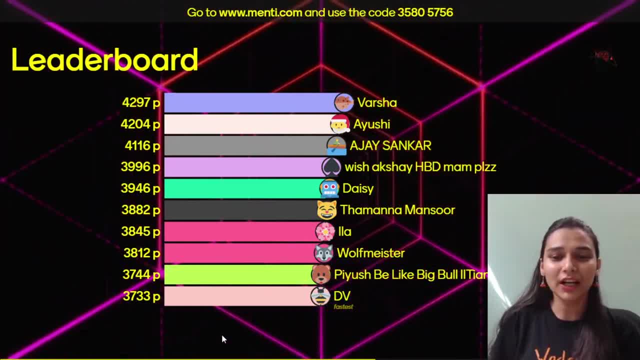 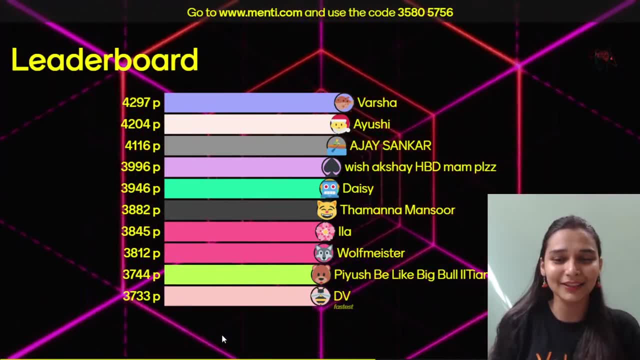 Varsha on the top now. Second, Ayushi Ajay. Then we have Vish Akshay. happy birthday, Beda. I did that, Akshay. happy birthday to you, Yes, And stay happy, And you don't need to attend Menti today. 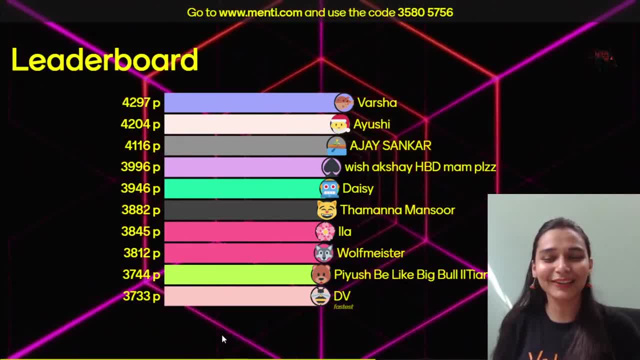 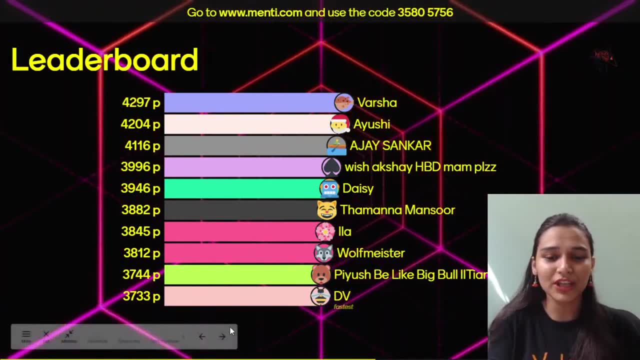 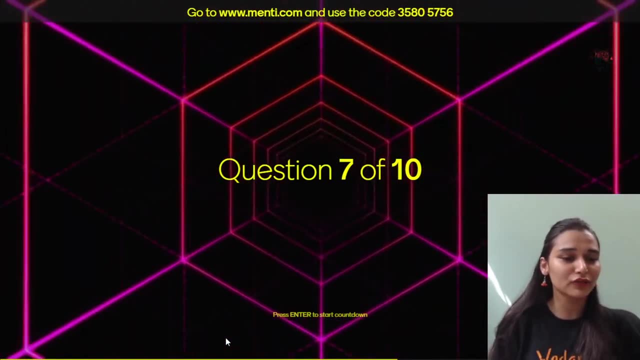 Okay, you can just take a chill pill. What are you doing here, Ma'am? I am here to check my IQ. Daisy and Tamanna again here, Ela Walsh, then Piyush And Devi is fastest there. Amazing, Very good Warriors. try it again. 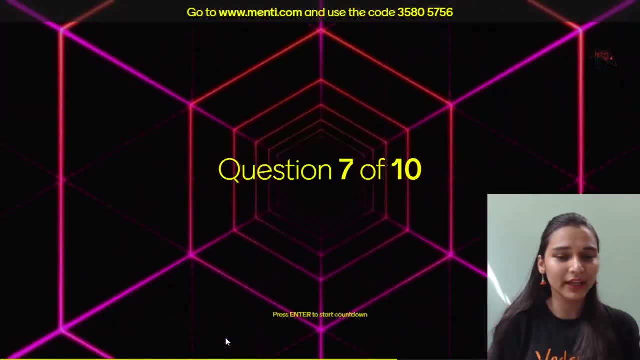 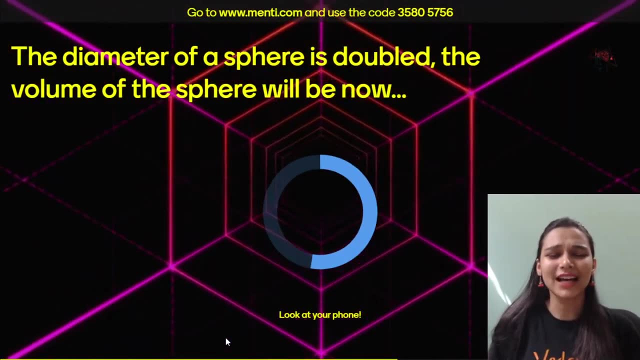 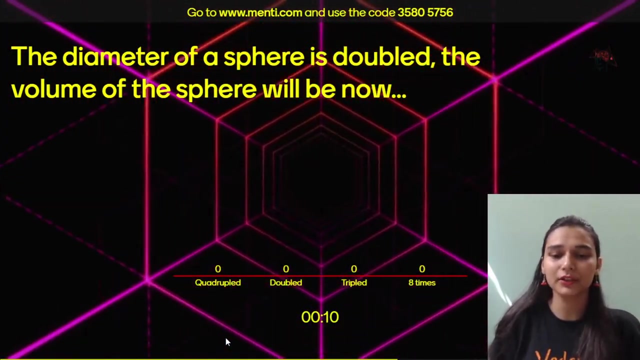 Maybe your internet is not working fine. Yeah, Seventh question: Get ready, And there we go. This is very easy. The diameter of a sphere is doubled. The volume of the sphere will be now Quadrupled, doubled, tripled or eight times. You guys know the relation. 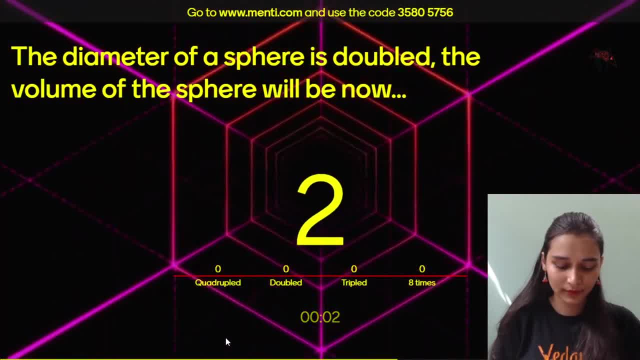 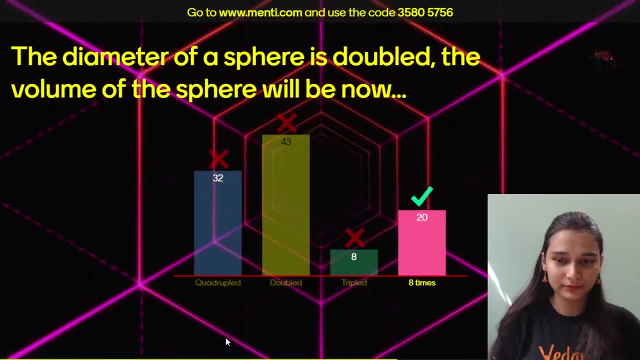 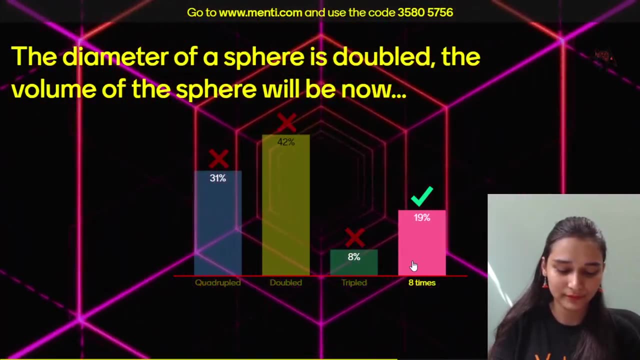 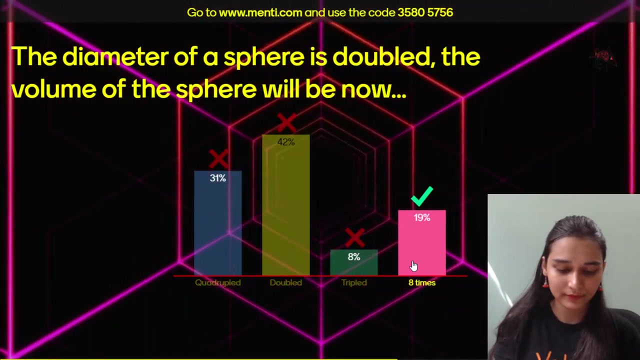 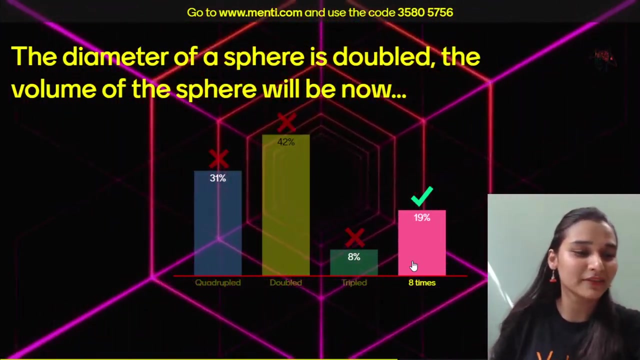 I am very sure. Okay, What? How did you do this wrong? Even I know this. Come on, tell me the formula of volume of a sphere. Yes, I can see. Tell me the formula of volume of sphere 4 by 3 pi r cube. Okay, 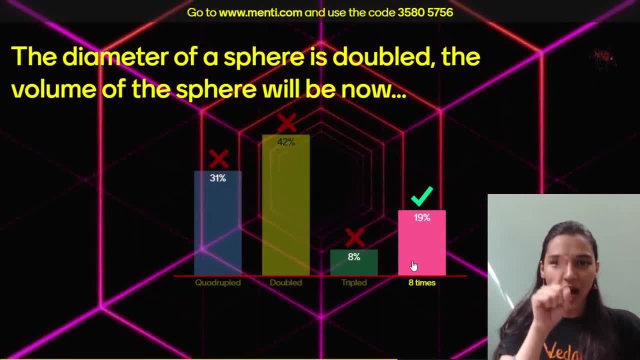 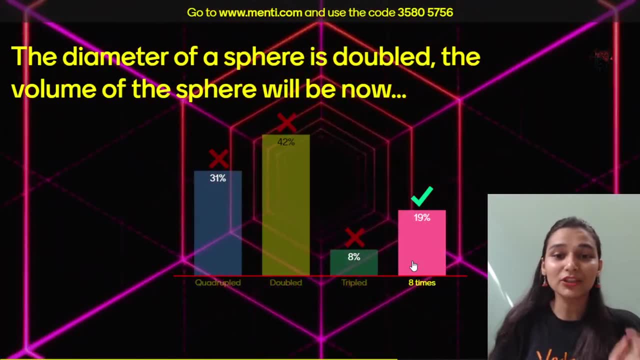 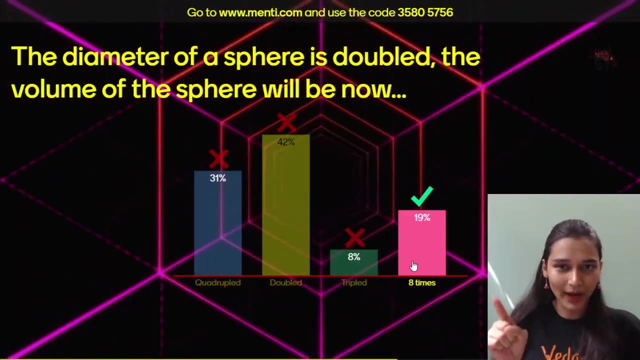 So I can say volume is directly proportional to r cube. That is right, Volume is directly proportional to r cube. Now it is saying that diameter of a sphere is doubled. You have doubled the diameter, So radius is equal to twice of. You can just take that, Okay. Yes, diameter. 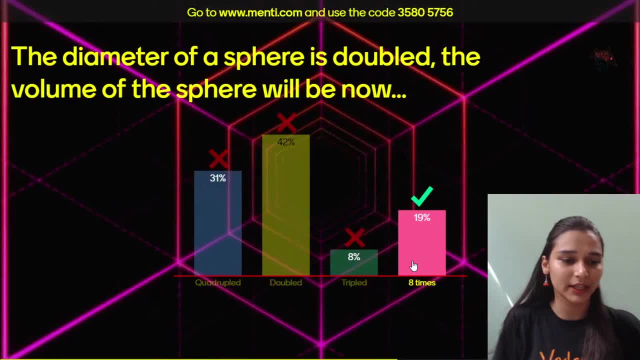 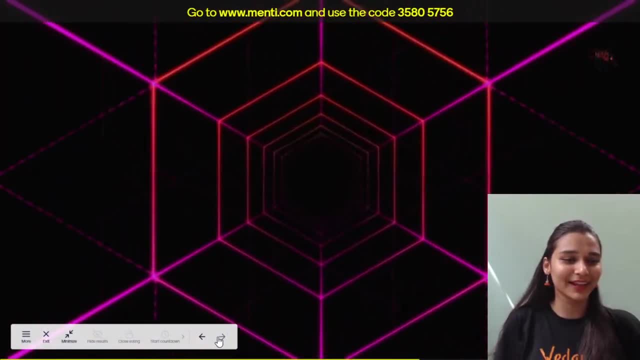 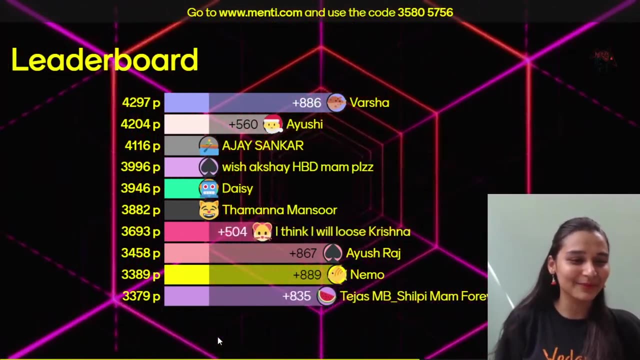 And then you have to double it. You have to make cube of that also. Okay, Yes, Okay, Come on. Let's go to the next one. Ma'am, don't you know maths? Okay, Yes, Did you see? Ma'am knows maths as well. That is the only thing you have to keep in mind. 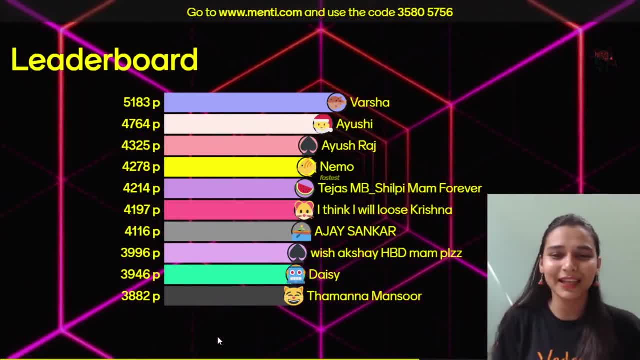 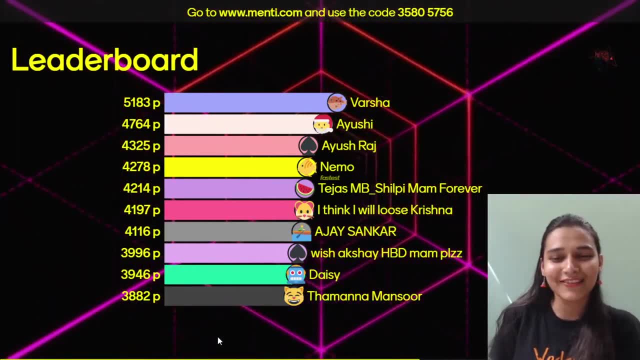 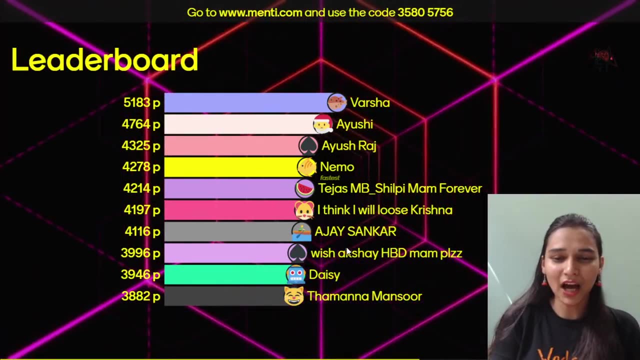 Volume is directly proportional to r cube. Then substitute the new one, You will get the answer: Varsha Ayushi. Then Ayush Nemo, Encounter inating, Believe it will be. this time Amazing. Tejas will be ma'am forever. Wow, Tejas forever. Yes, I think I will lose Krishna. 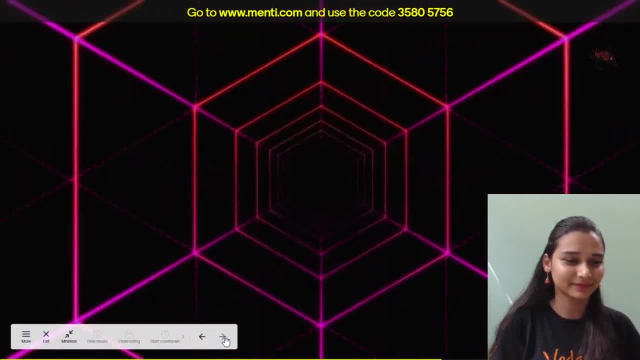 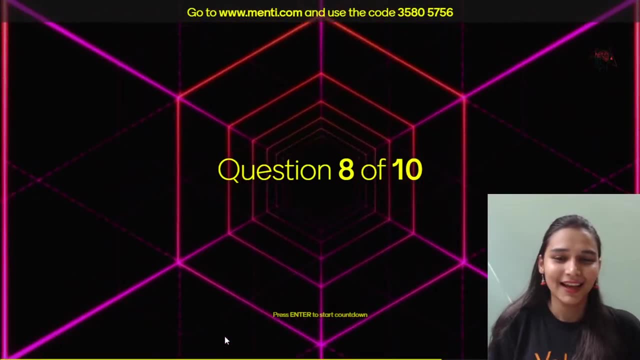 Okay, Then we have Akshay, Then Akshay. Happy birthday Daisy and Tamanna. That was amazing, Shashi, I got hundred marks in maths in tenth standard. Yes, Okay, Eight one. And for information, I got 95 in 12th. Excuse me, I forgot now. 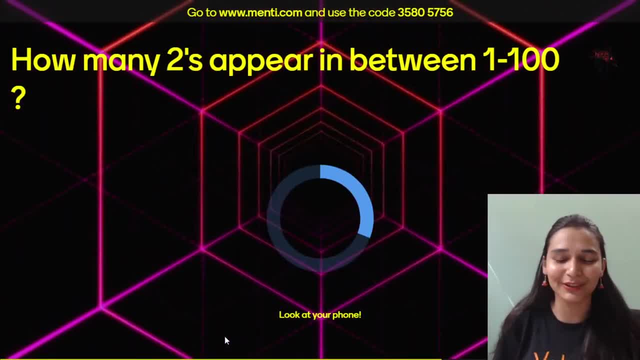 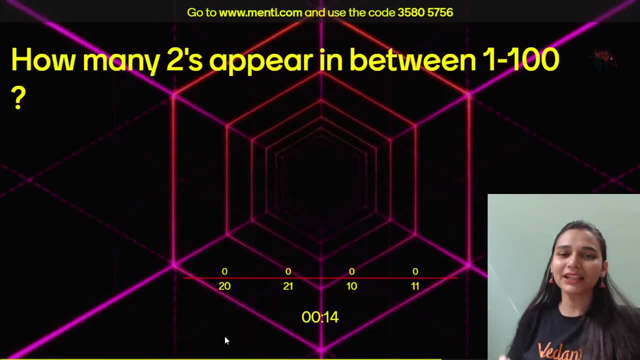 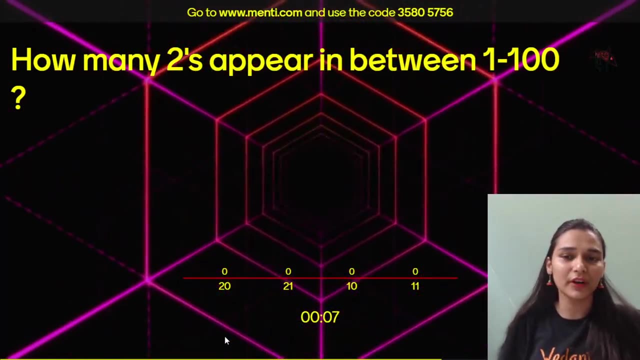 Practiß. Wait, Take it. My computer has not started. work at 11 o'clock is like okay. sometimes math becomes difficult, but it is one of my favorite subject: how many twos appear in between 1 to 100. so how many two digits, like how many times this number appears. 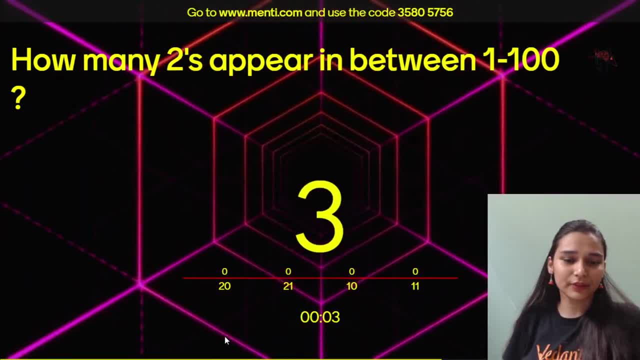 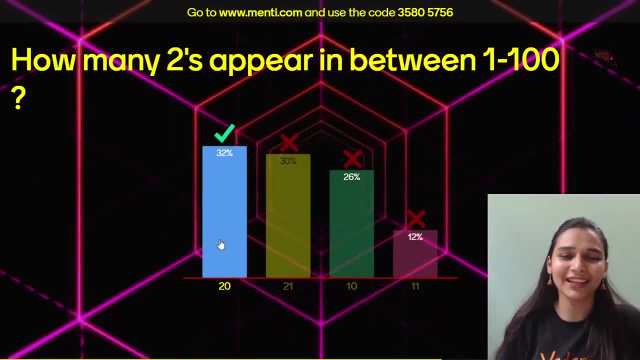 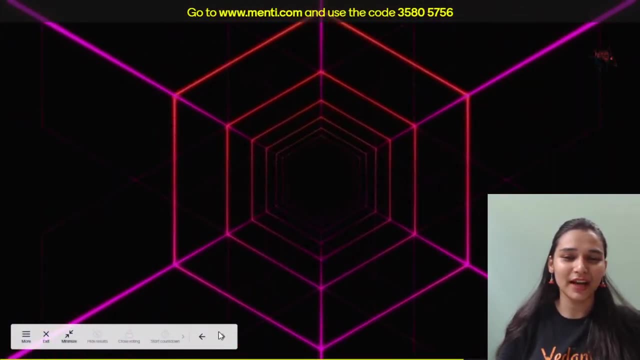 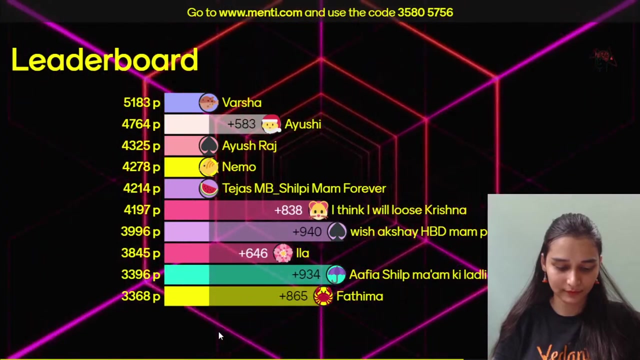 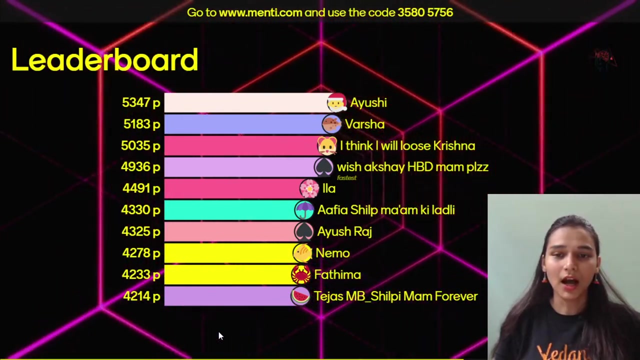 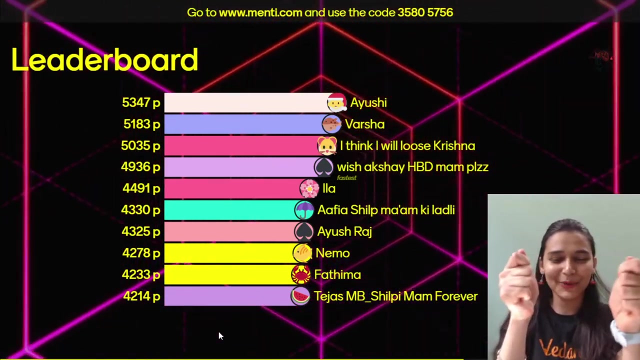 in between 1 to 100. yes, go for it. come on, are you sure? 20 times now check it out how. just let me know in the comment section. okay, chalo, let's go to the next one, ayushi, on the top. now i will just do this to your cheeks. 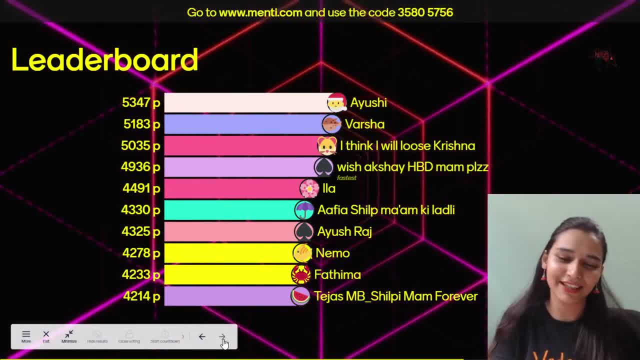 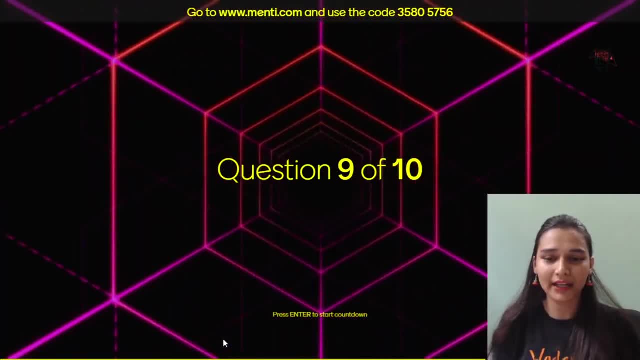 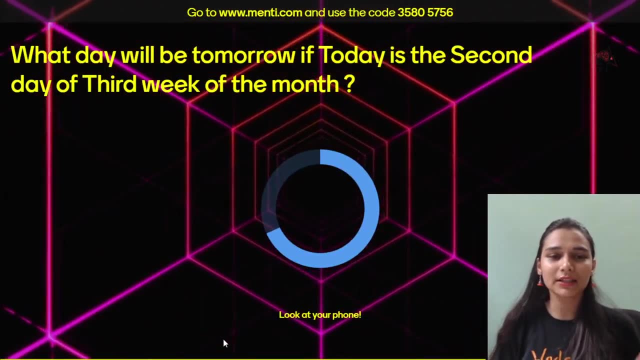 amazing guys. you people are actually doing brilliant. still, we have two more questions. like the video and get in the ninth one on your screens. there we go. the question here says that what day will be tomorrow if today is the second day of the third week of the month? 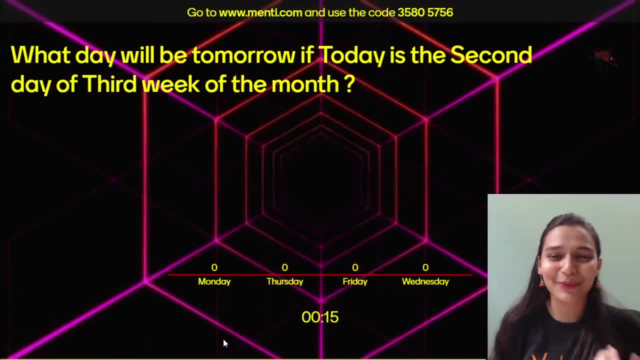 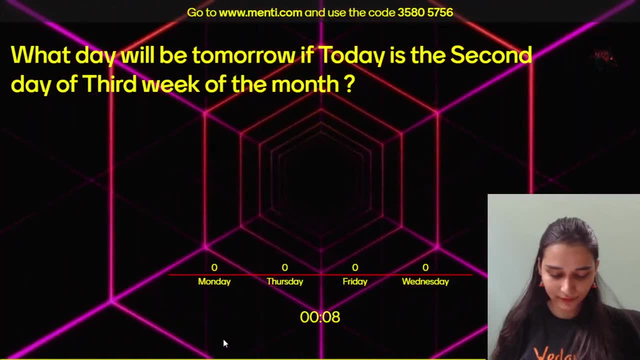 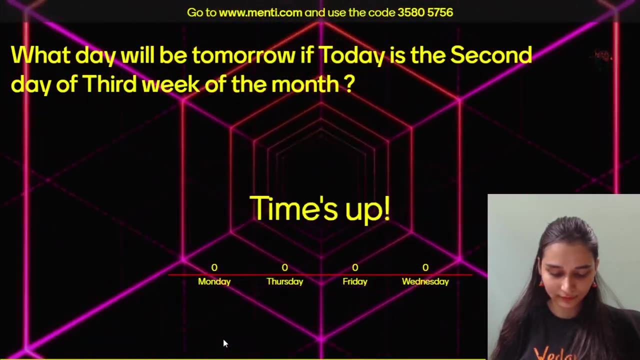 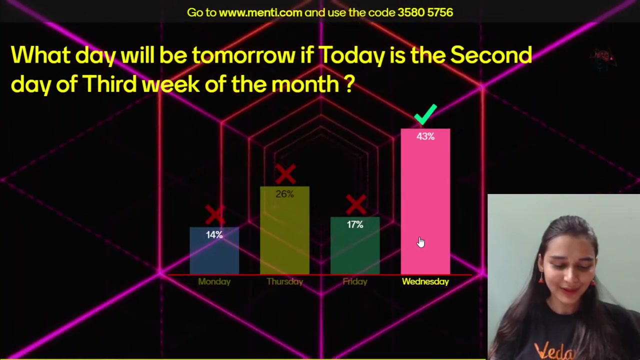 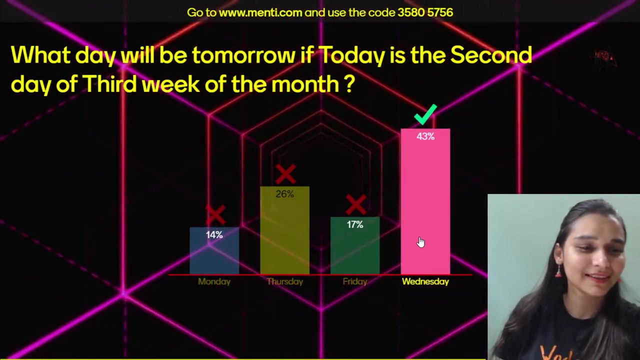 let me take a break. when is day, guys? how you have done it. i mean, how did you guys do this? tell me honestly, like i actually need to clap for you now. huh, that is actually very amazing. mikhail 152 likes we have achieved. that's amazing. 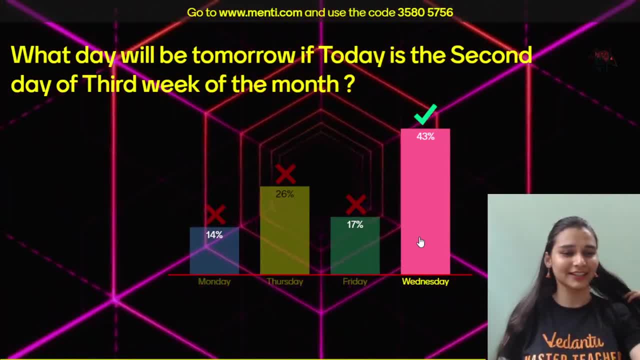 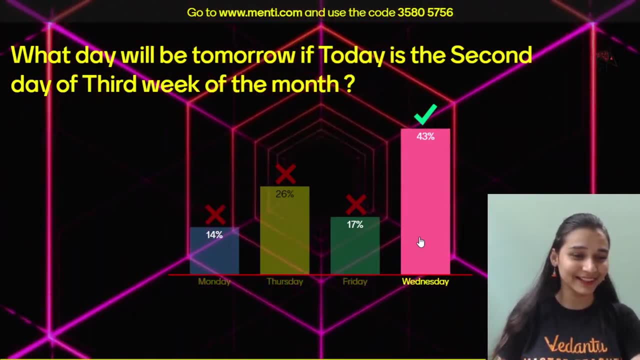 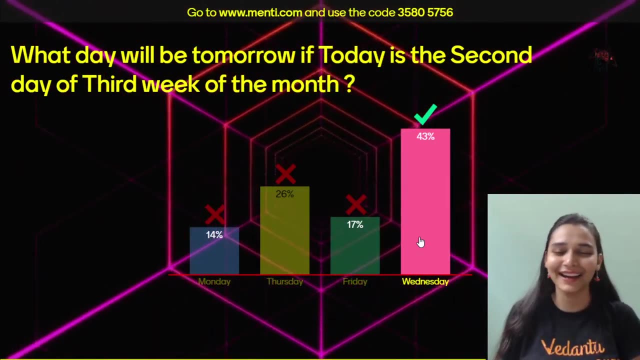 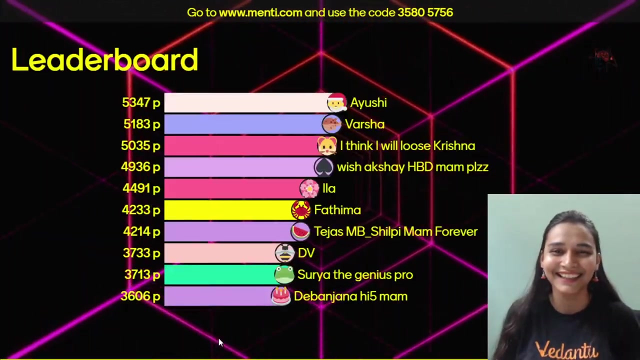 khatam hone ke baad, 200 also. we will achieve, i'm very sure. yes, yes, shashi, that's right. true, true, true, ma'am, dema, mein google hai. really. yes, priyal 30, first day, and harsh sir would be enjoying right now. achintya, i don't know, i really don't know who like. who is the founder? like for the mentee? yes, it's okay, shri, koi baat nahi, we will try again. 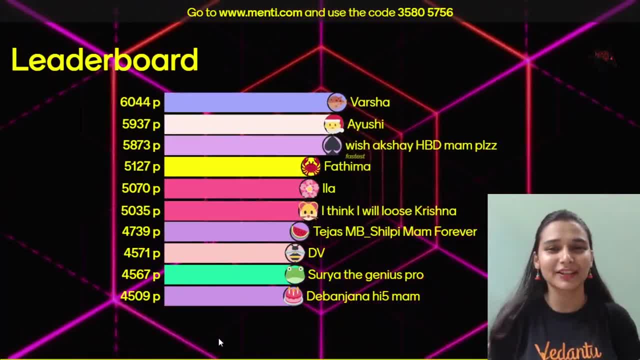 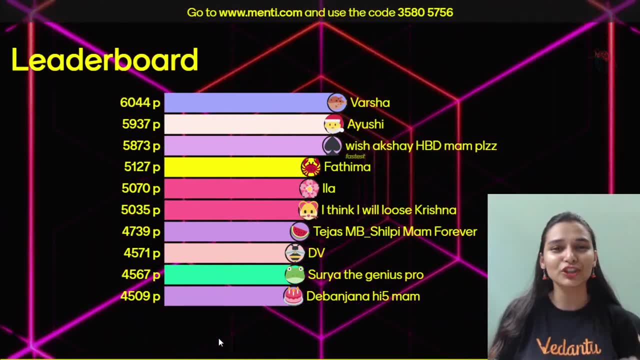 if you like this session, i will come up with more such sessions. jaisse, we have iq aise hi vi are having other questions as well. eq bhi hota hai emotional questions, so how you actually handle that thing. we can have a session on that also. 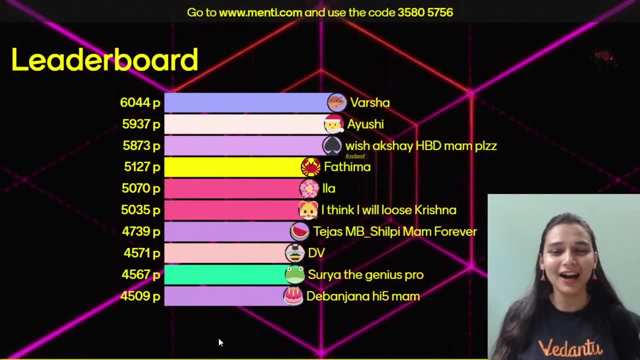 okay, then okay, varsha, ayushi, akshay, fathima, eela krishna, tejas, dv surya and nibanjana, high five, beta chalo. the last question is coming in. varsha has taken a break from diwali. daaai baiyai bhi hi bhecht hai. bhai hai siya ho jobin hai ji na ребята chalo last. so aakassha is giving an emailit to me by mail. 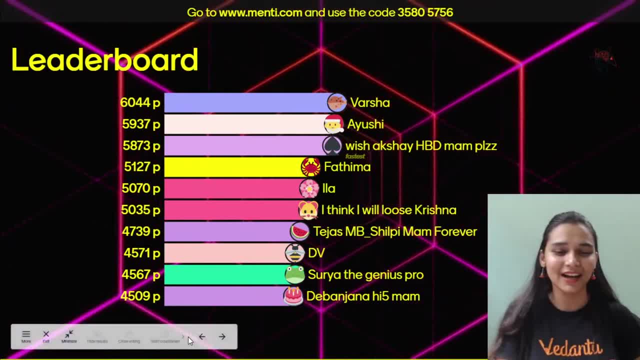 ふكرا kau ki ki teenage sir isостоin ke share ke parfaitования of major budget fees. to na, to jo hell, we have even time. tis a leaking surya acj grr me get andbrillays ai paaj sab ma hai ne weather gahi hu. 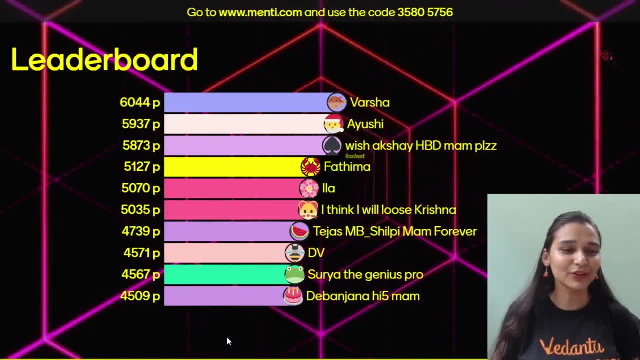 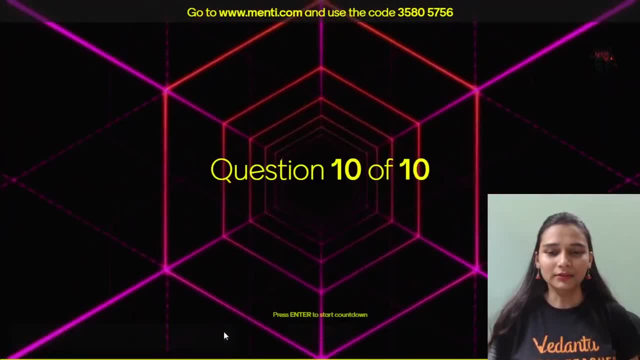 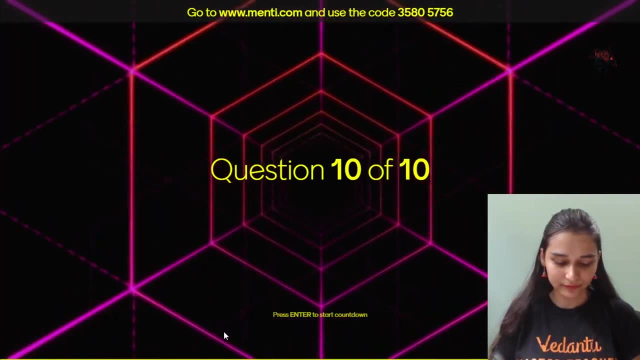 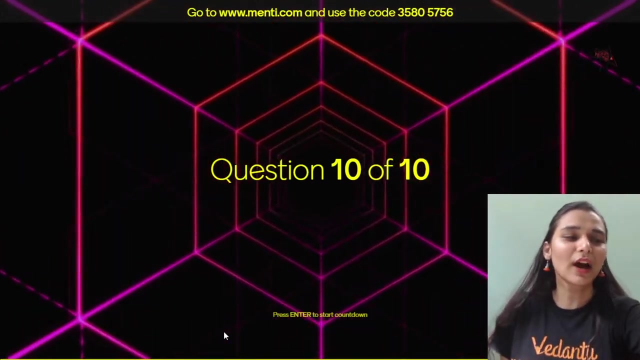 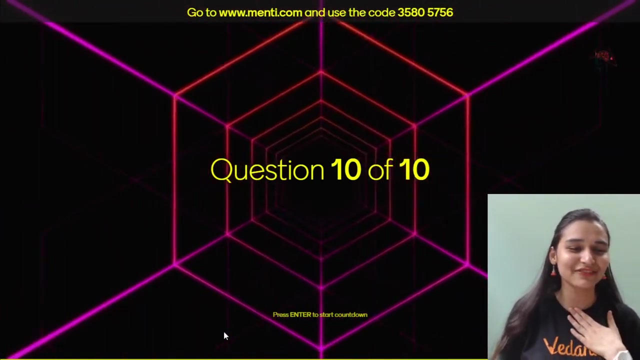 has taken actually a good lead. very good, we have the last question now. are you all ready? one more question is there? yes, keep on trying, keep on trying. ready some blue hearts in the chat box please. like blue hearts, they act as a fuel. yes, when i say fuel, then you have to start spamming with the blue hearts. 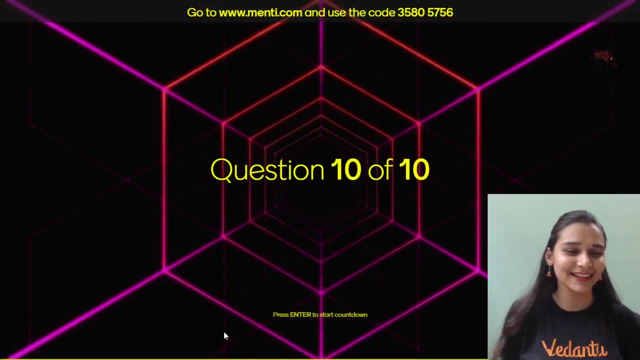 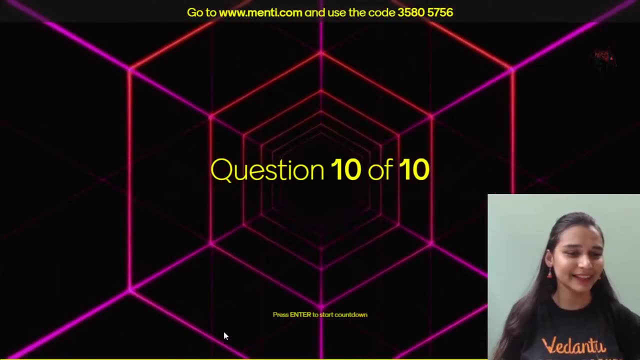 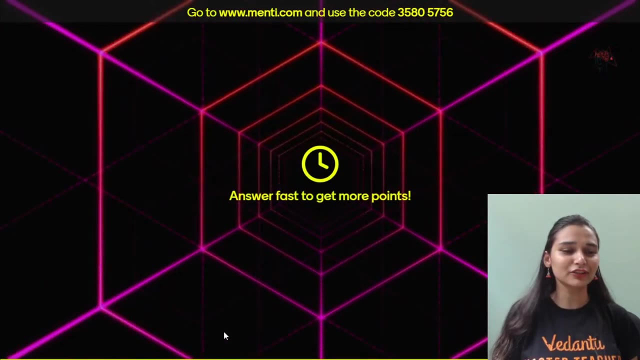 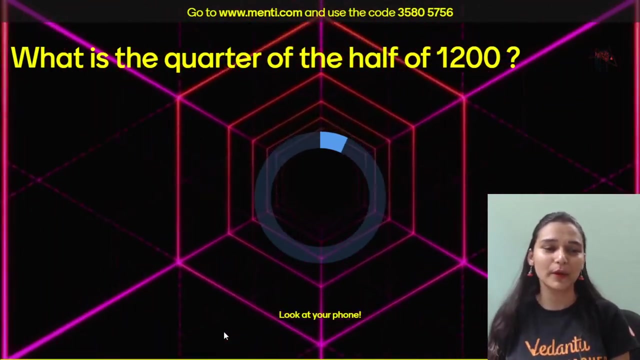 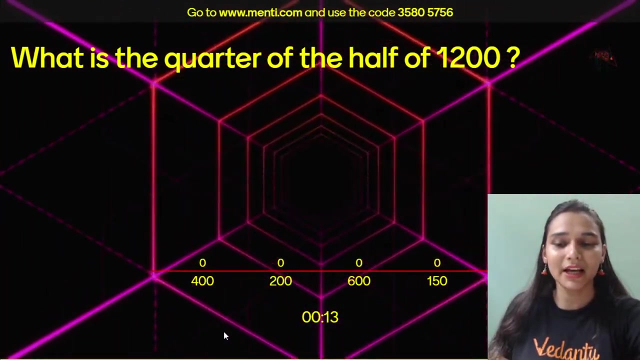 it's time to give fuel to the engine. yes, very good, that's. that's like a good student. hi, nandini, taken your name. yes, awesome, 10th question on your screen. guys, join in the 20. still, you have one chance. what is the quarter of the half of 1200? quarter of the half of 1200- 400, 200, 600 or 150? 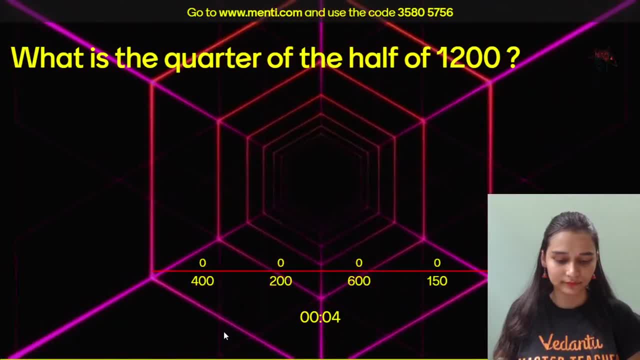 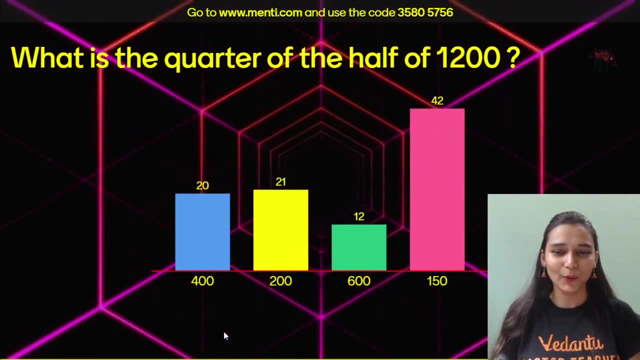 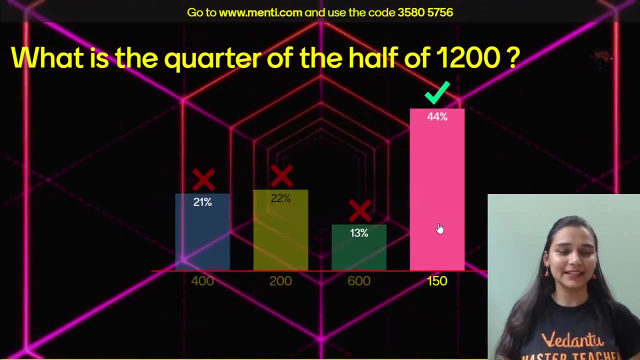 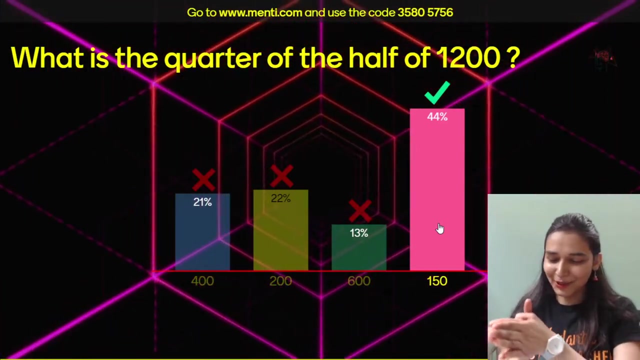 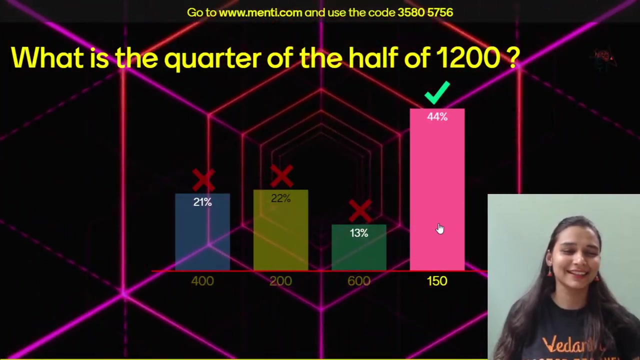 yes, and i can see now. that's amazing. what do you think? yes, i understand. what do you think? yes, this was the easiest question yet. only 44. 1, 4 of the half of 1200. 1, sir, would be 600. 600 divided by another�, both will be 30 000 water to sobie unke lade Le Truck worsh start should go till ca n l. you are a loading Gun Club. now let's see who will get a loading gun club. ki se mile gau loading gun club. what do you think? yes, this was the easiest question from chap. know who will get a loading gun Club. what do you think? this was the easiest question from chap. know who will get a loading Gun Club? what do you think? hei was a loading gun club. yes, yes, this was the easiest question anymore. only 44 %. quarter of half of 1200. half of 200 would be 600. ہن فارقرایی yn commenتي. 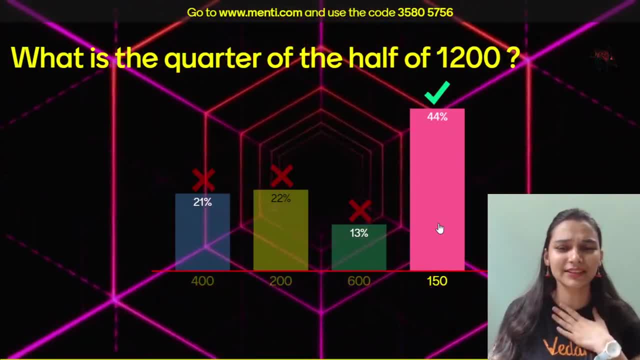 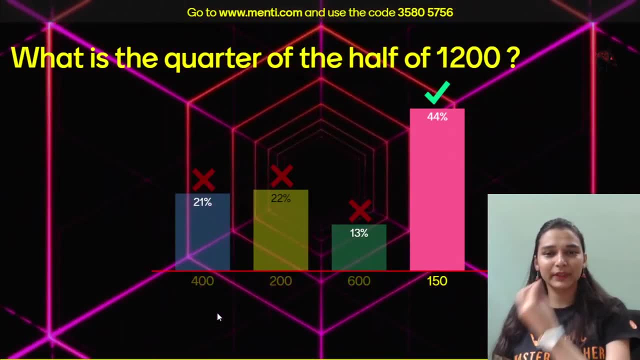 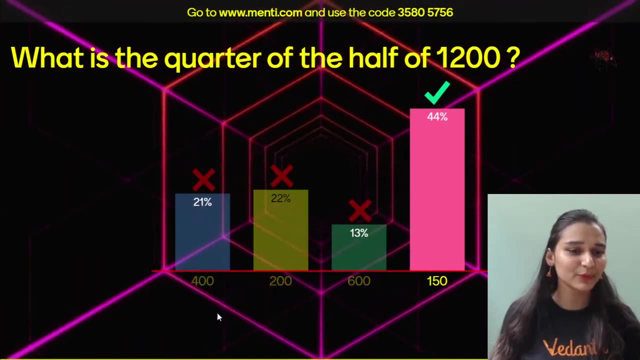 are you able to get a loading gun club quarter of the half of 1200 ni klaabato briefing ni. the half of 1200 would be 600, 600, 600. divide the four, say that will be 150. that was easy, clearly saying varsha says: okay, let's go. 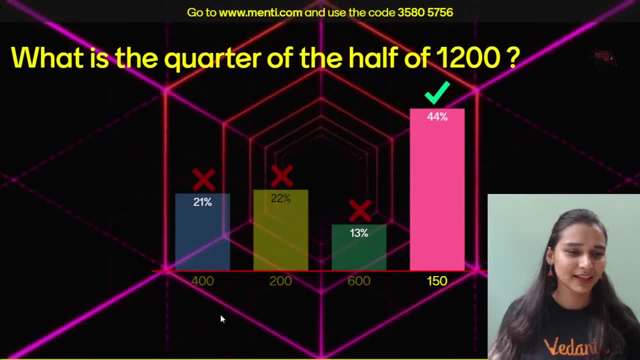 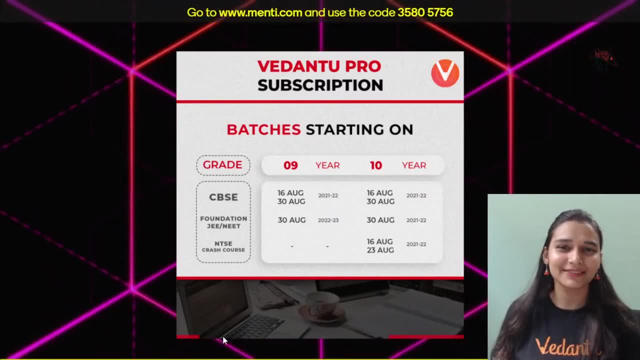 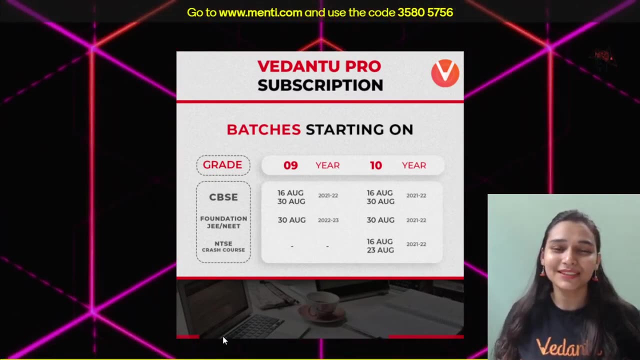 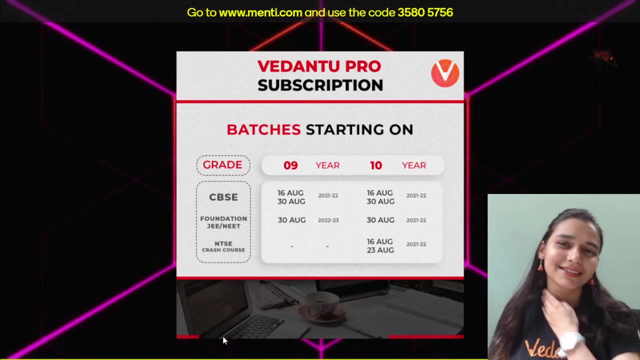 and see muskan. okay, i can change. i can change the mentee position, provided you guys like, everything has a price, yes or no? do you agree with that? everything comes with a price. so if you, you know, give me some sort of bribe, maybe i can change the answers on the mentee and i can make you win. but 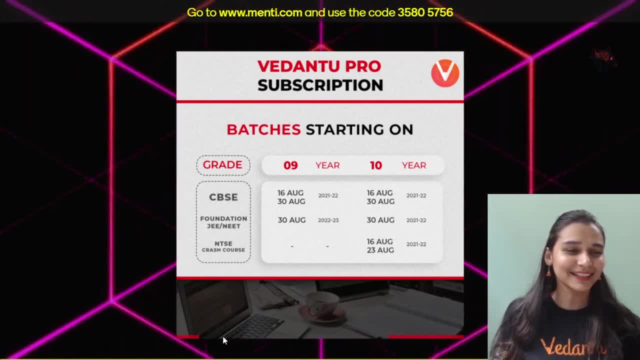 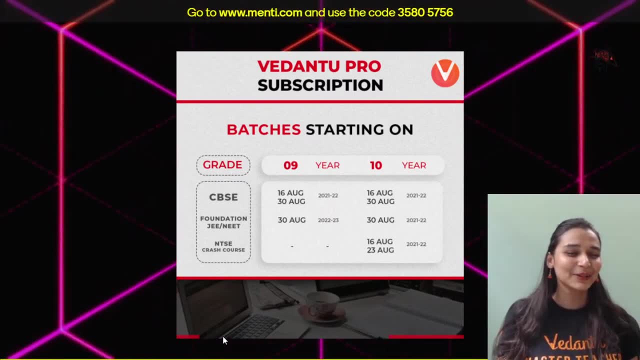 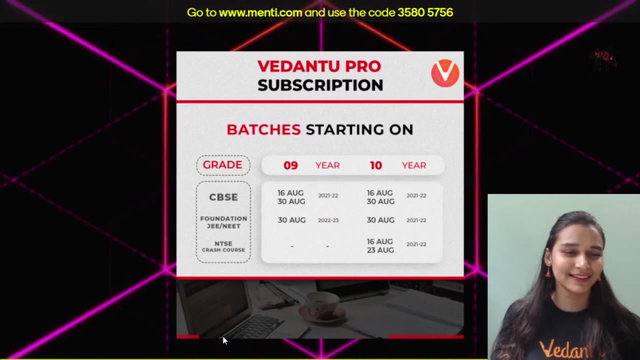 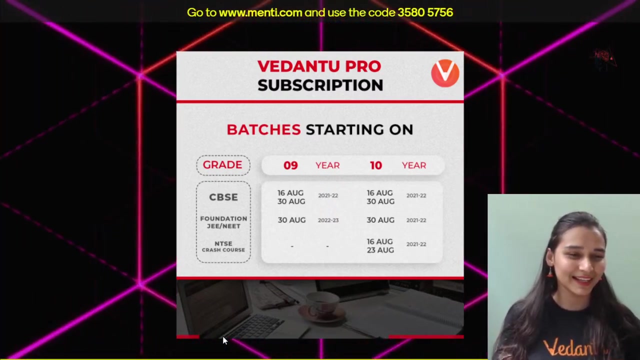 i should get something for that. they just saying: ma'am, okay, janki is also ready for the offer. muskan is saying: ma'am, i will send the blue hearts in your every session. i can think about it as well. blue heart okay. ma'am okay, i will give you oreo cakes made by me. number now, my heart is melting. 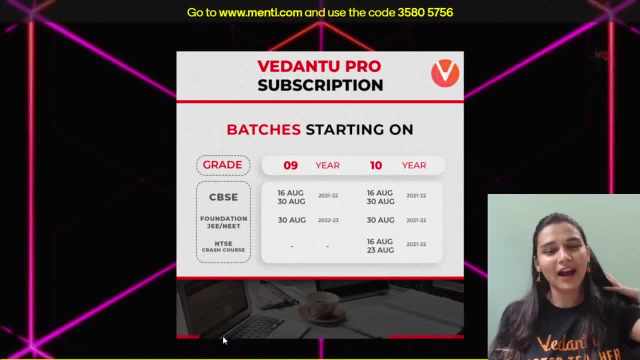 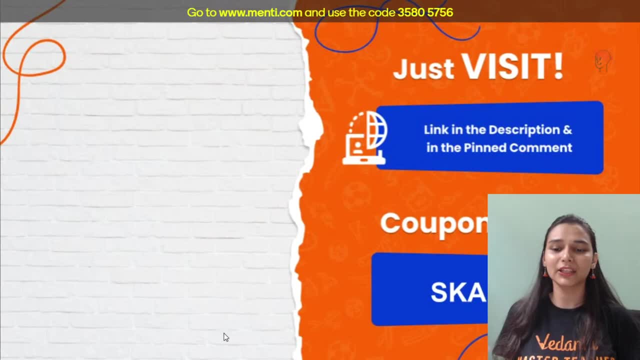 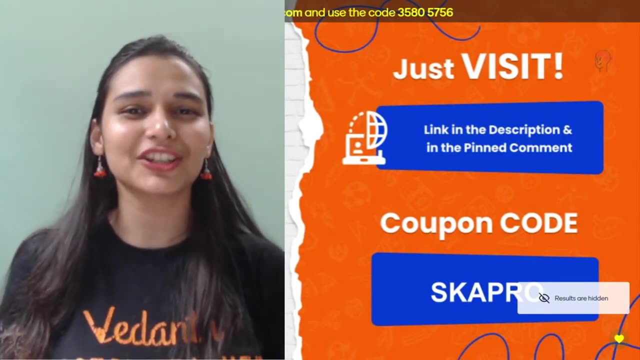 okay, ma'am is only kidding, why? no, like nothing can replace your hard work and your iq for sure. so yeah, again reminding you, if you want to be in my pro batches for one month, then you can go and simply apply sk a pro that it should be kaushik army. so army and 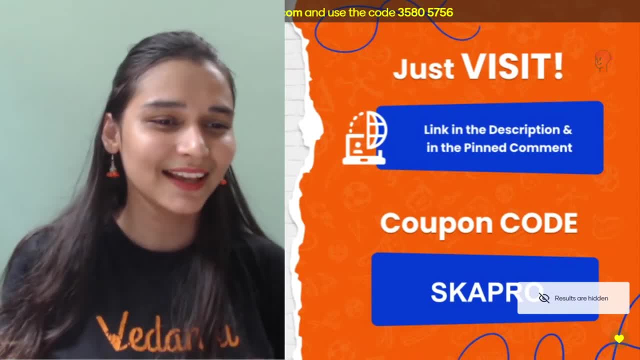 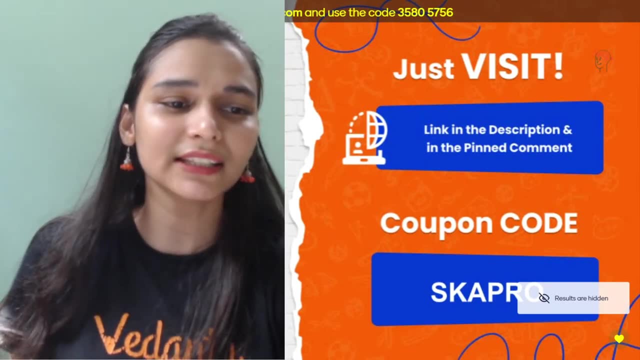 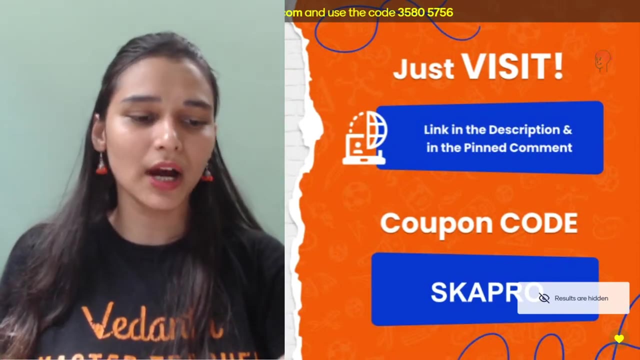 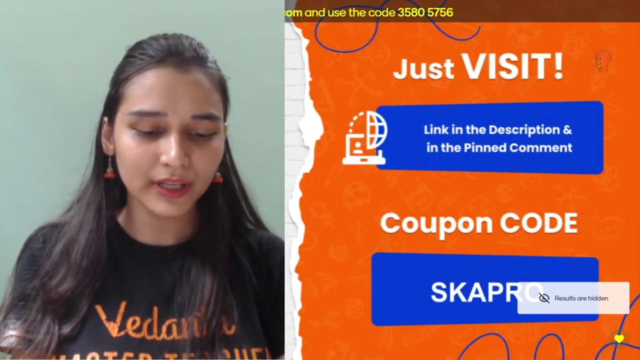 i believe my qatarian army would be there. yes, i will give to ananya. sir, in the chat box, two people can make two bicycles in two hours. how many people are needed to make 12 bicycles in six hours? so i want to know the answer from you in the comment section. okay, 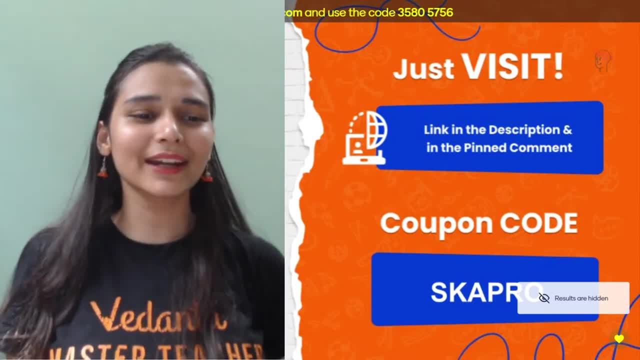 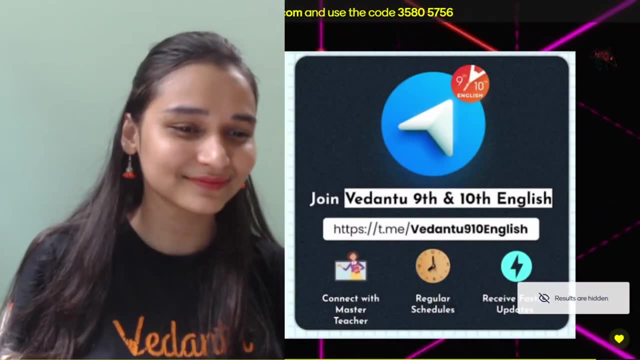 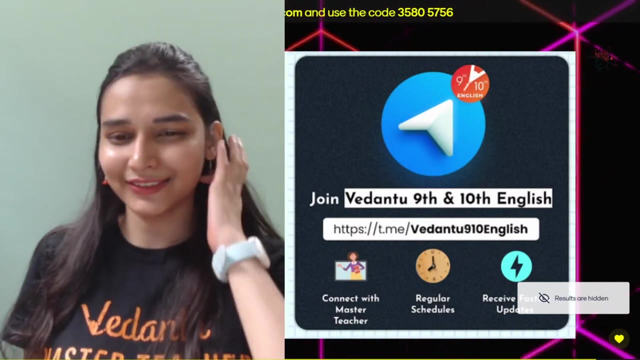 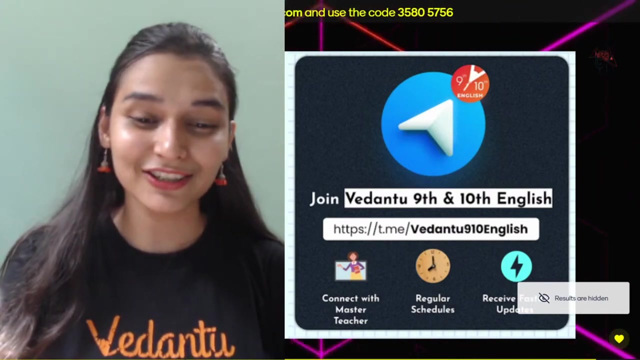 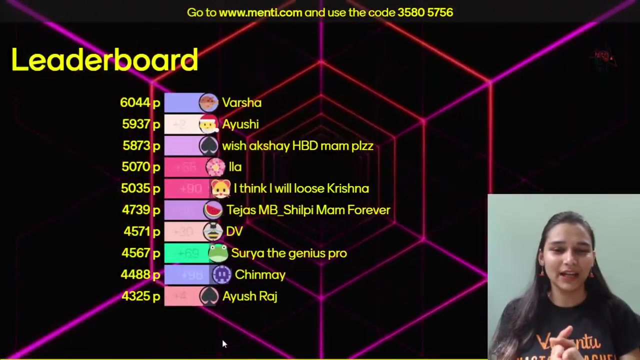 okay. okay, i can see in the chat box. i will give you a cheese maggie, okay. so now, that is actually a very difficult call for me to decide. let's see the leaderboard and this clap is coming. oh my god, this is a very difficult call for me to decide. let's see the leaderboard and this clap is coming. 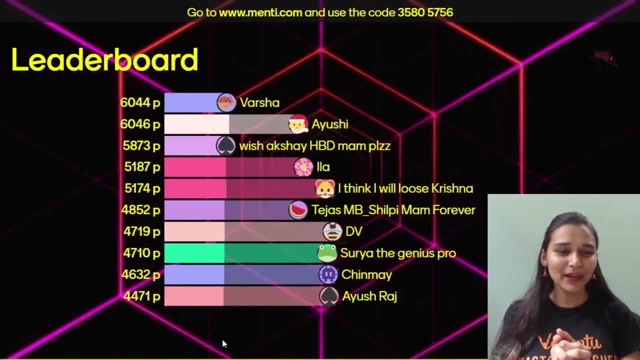 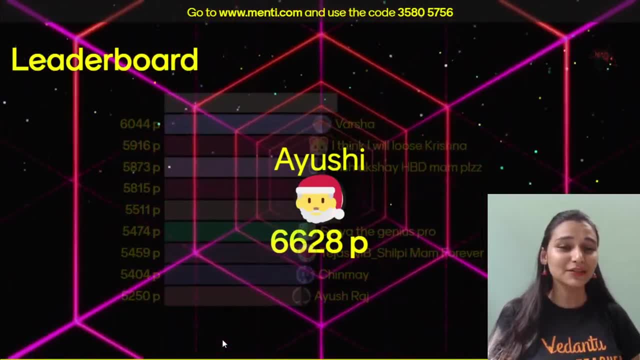 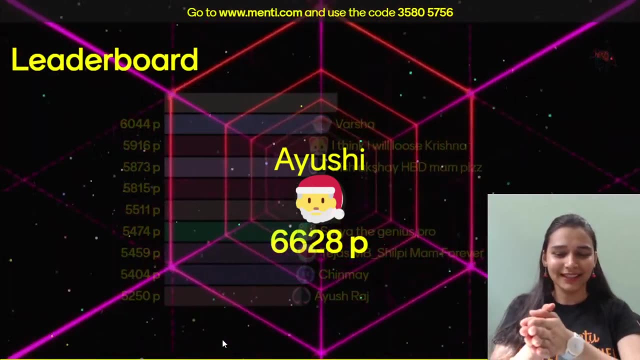 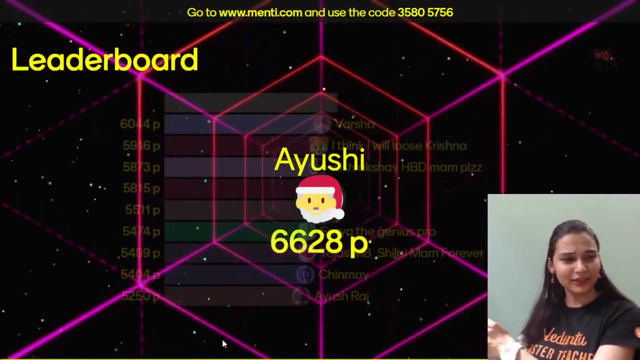 So, Varsha, like you marked that wrong. jaldi, jaldi mein over X. no, like no, ma'am Ayushi has done that and the point difference kaafi hai. that's amazing. now it's like the loading gun machine ki clap ki baari hai, and how it starts. we have to fill the bullets first, chike, I will put: can you see my hands, haan? now you can see that. 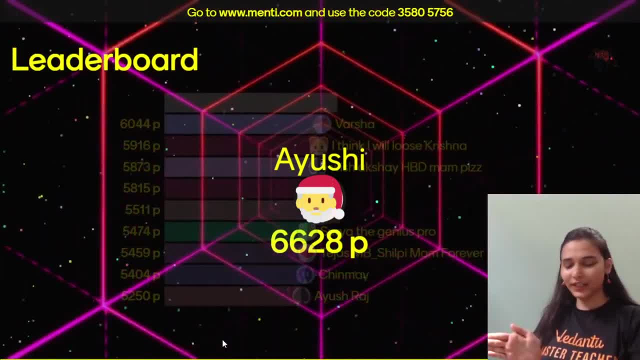 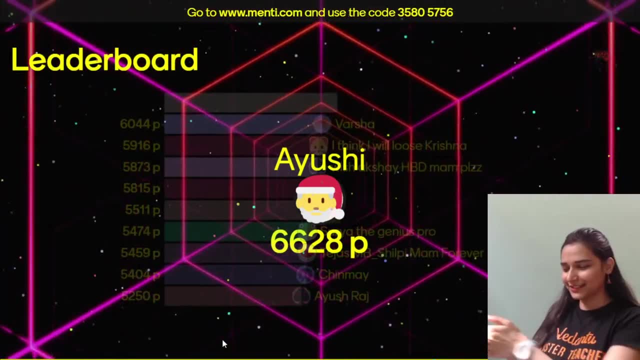 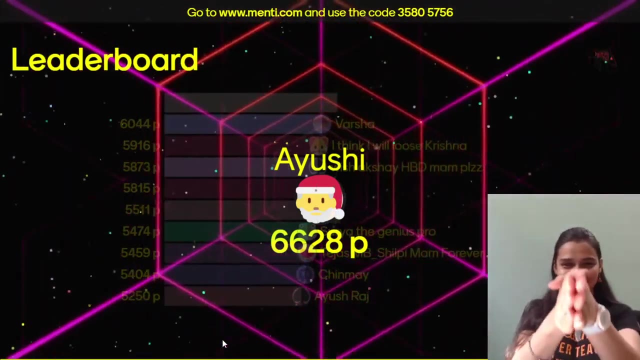 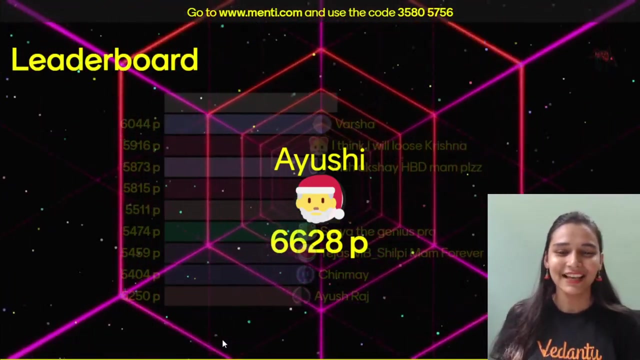 ok, so we will fill in the bullets first, and once the bullets are ready, it's time to load the gun. yay, that's how it works, and twice. ok, Ayushi, that was for you. I have to think of more such ideas. yes, so next time we will have a bubble gum. clap chike, jo bhi next session hoga. we will have that. 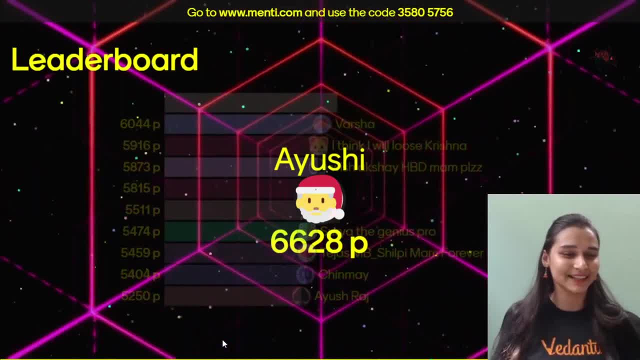 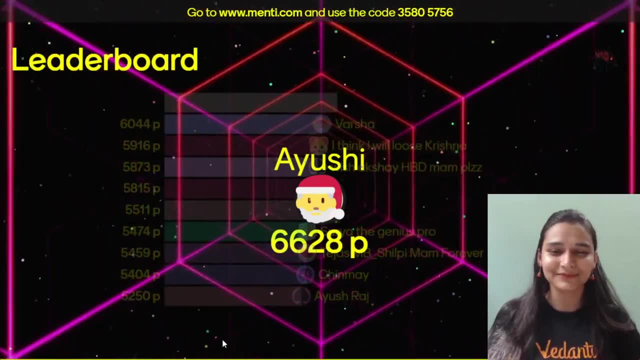 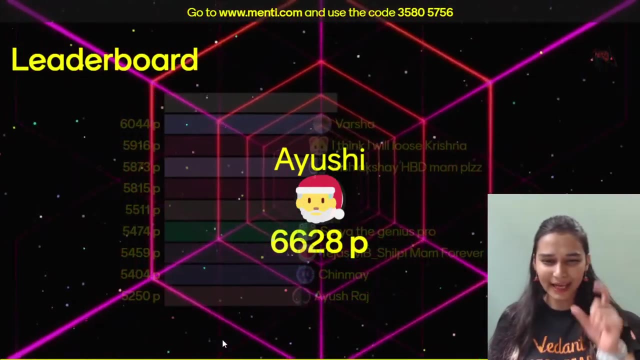 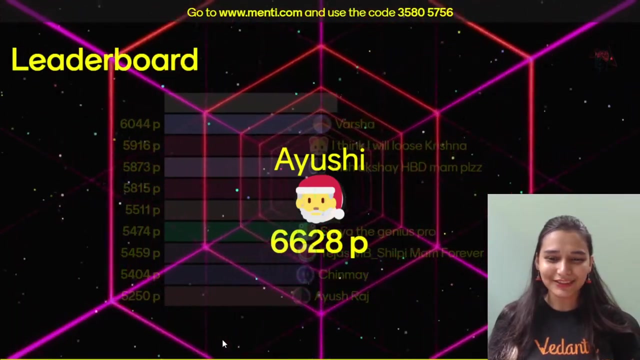 yes, Anjali, 11th position, that's amazing- 17th. so each one of you has done an amazing job. and Ayushi, like you, got the first position in like IQ wala. that was amazing. and still I can see Varsha is there, Krishna, Akshay is there- some names are hidden there- and I can see Genius Pro is there, Tejas is also there, Chinmay and Ayush is also there. 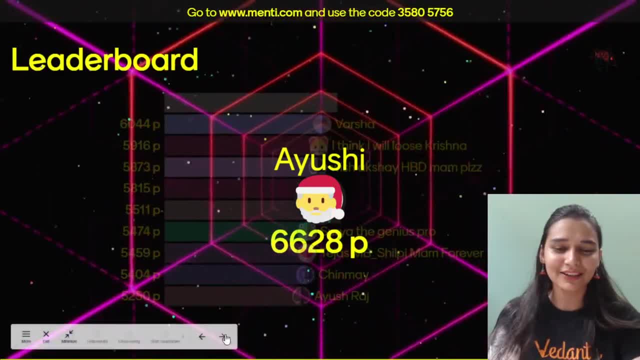 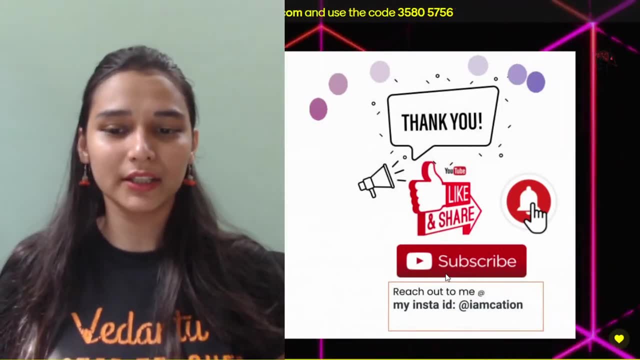 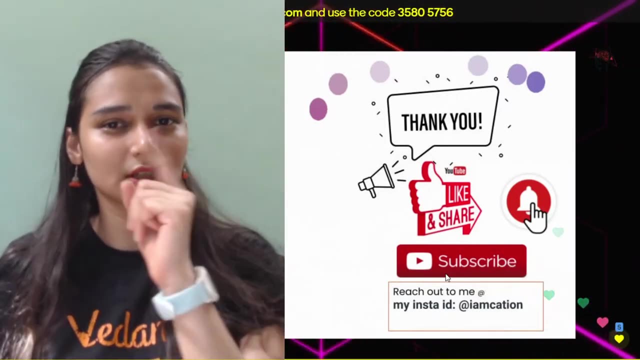 so you, all of you, have done an amazing job, guys. I am actually really proud of you and just telling you, if, in case, you want to reach out to me, then I am available on Instagram. I am Kitanis, my ID- and do not forget to tell me the answer in the comment section for the question which I gave you. ok, for that. labor wala question. yes, 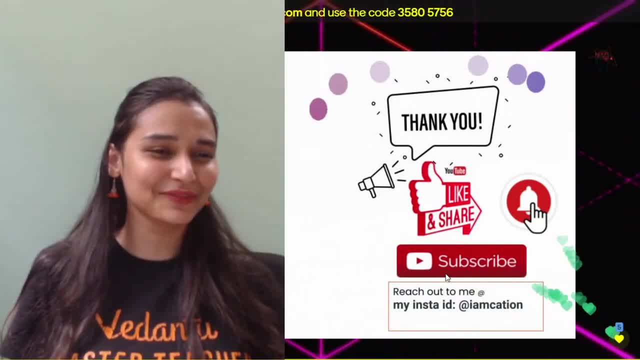 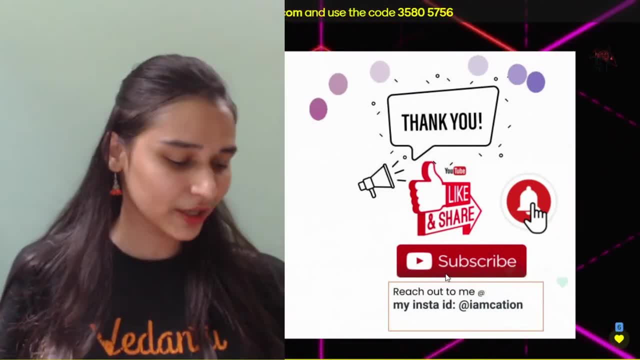 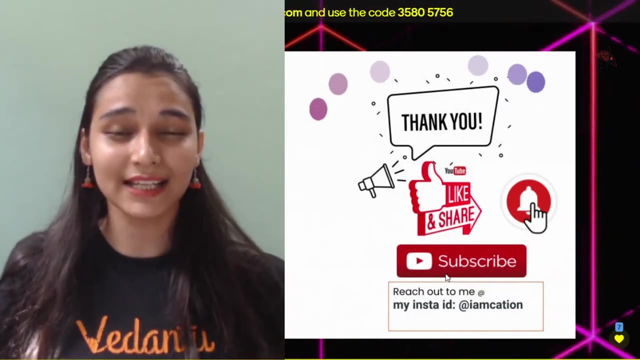 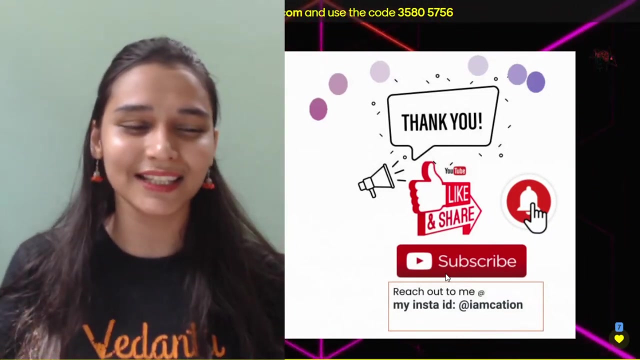 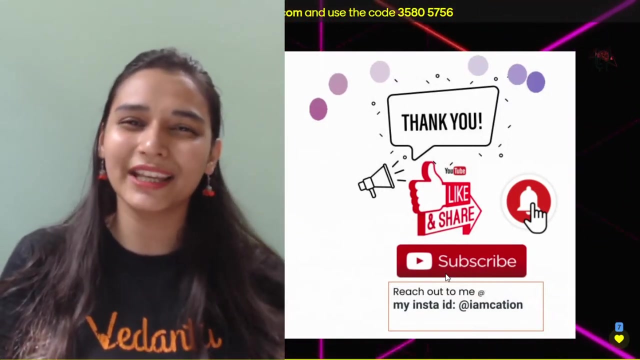 Pashpan ki yaad aagayi. ok, chike. so, Tejas, why are you sending broken hearts, beta? it's like it's ok. if not the first position, that's ok, yes, ok, so do. let me know your IQ position in the comment section and ma'am will see you next time. and if you have any more ideas- like ma'am- we also want to have a mentee on this topic- then you can let me know in the chat box, ok, like in the comment section, basically. so ma'am will see you next time. till then, take care, and I will pass on your wishes to Harsh sir. ok, so he right now would be enjoying, so we should not disturb Harsh sir, ok, ya, bye, bye, take care.